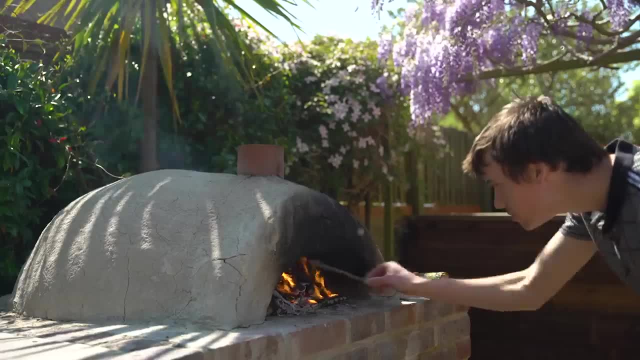 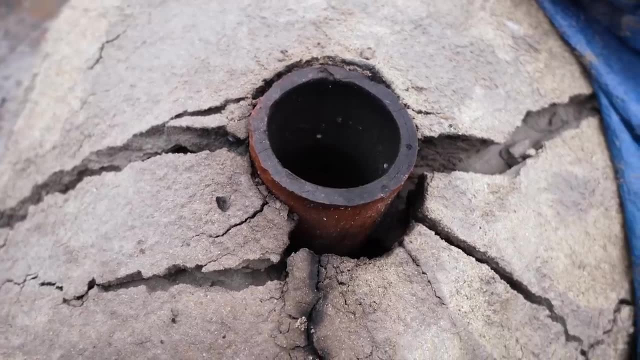 bit of damage to some parts of the garden. My pizza oven, which I so much love using in the summer months, got very wet this year and has actually collapsed, So I'm going to have to sort that out. After observing the mess that was my garden, I started writing up a plan. 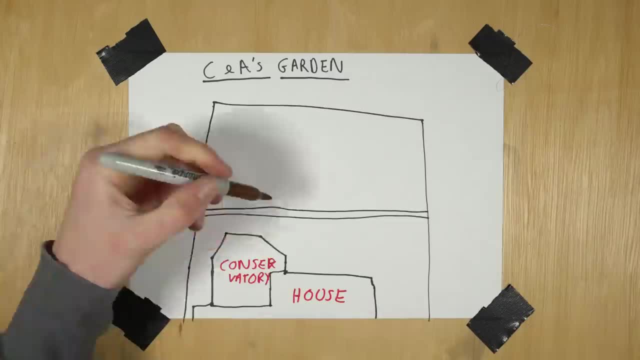 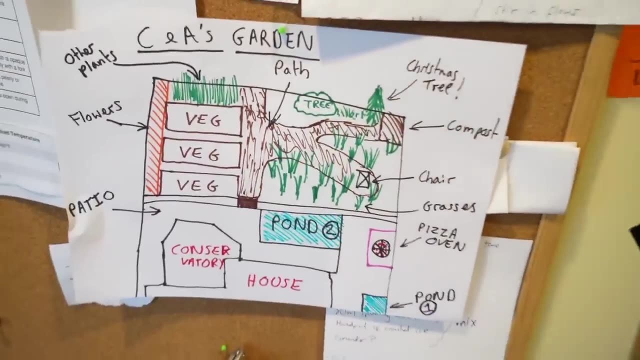 which you could describe, looked more like a five-year-old kid's drawing. I should point out that I live with two other people, so I couldn't just go digging up the whole garden. I was allowed a third of the space, which is 15 square metres. 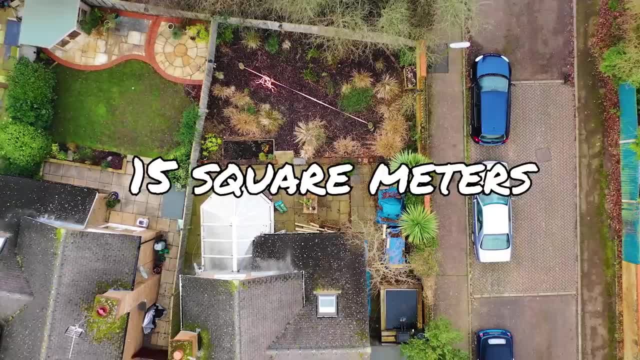 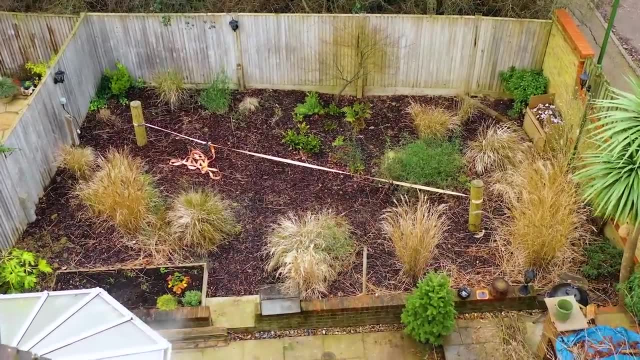 At the beginning of the year, I was told that I was going to have to start a vegetable garden At the beginning of the year. the garden had some grasses, some other plants in it and also a slackline like a balancing rope that I used every now and then to 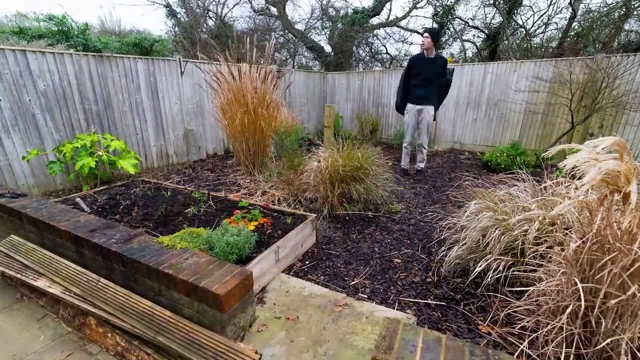 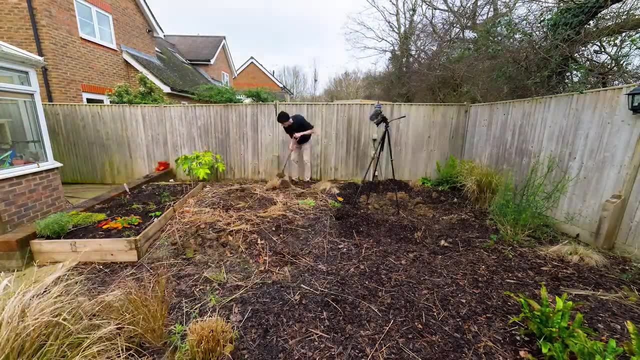 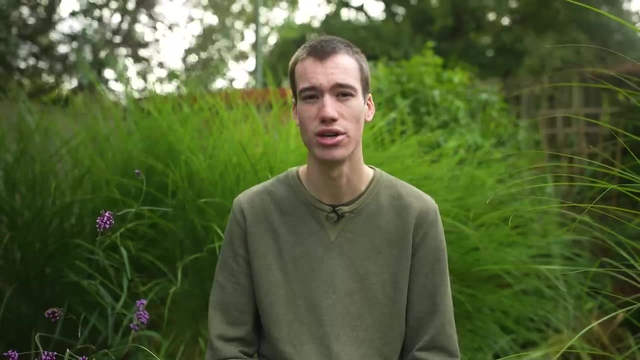 practice my balancing, But all that would have to come out Once the slackline was all dug up and pulled out. I then got to work digging over the patch. I dug over the garden and at this point I realised it was incredibly solid clay ground. 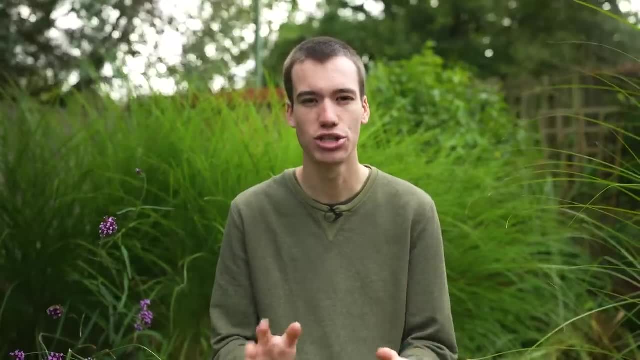 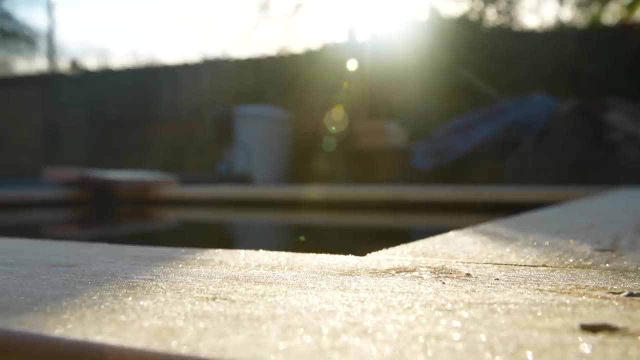 Which made it very hard to dig. So I was going to have to make some adjustments to that later on in the year. I would have liked to get cracking straight away and build the raised beds and get planting, but the winter was just relentless. It just went on and on and on. 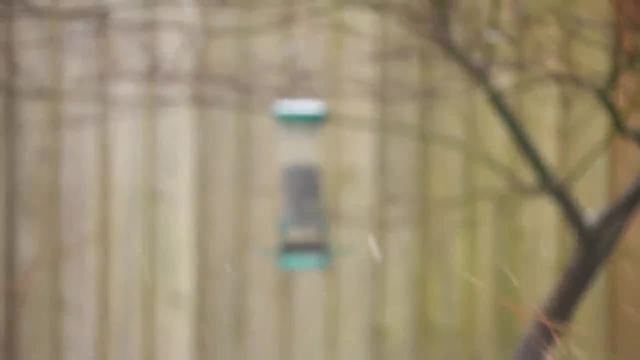 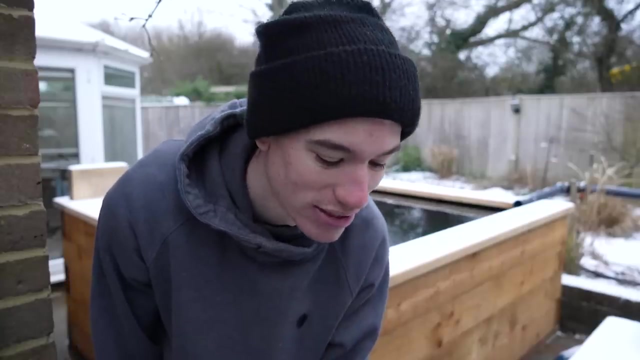 Well, it's such an exciting day for a southern English person like me because, as you can see, it's snowed. We can make some snowmen, play snowball fights and also eat the snow. So many fun things to do. 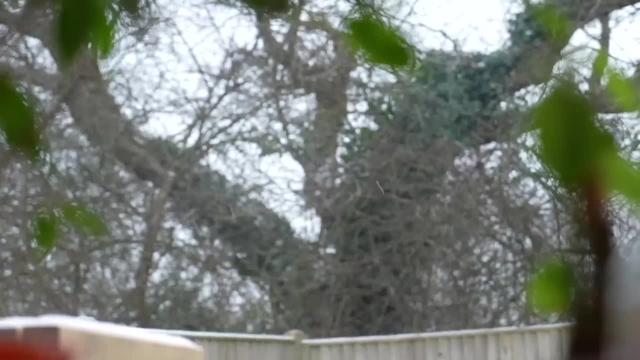 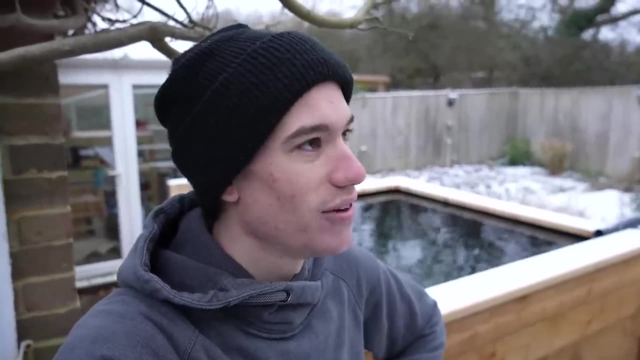 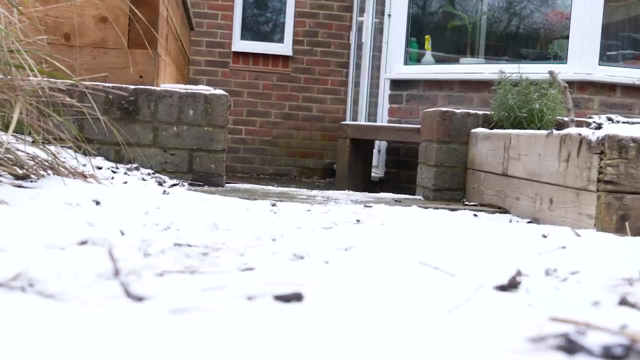 But it is annoying because it's mid-February now. My vegetable patch is going to have to be delayed still. I'll see you in a few weeks when it's 15 degrees and sunny and warm and spring is in the air. Because of the weather conditions I couldn't do much at all, But there was one job that I had. 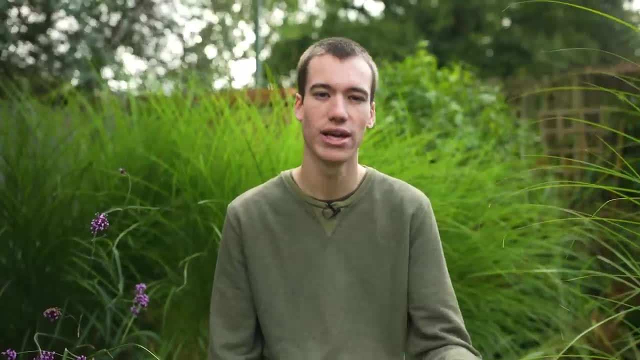 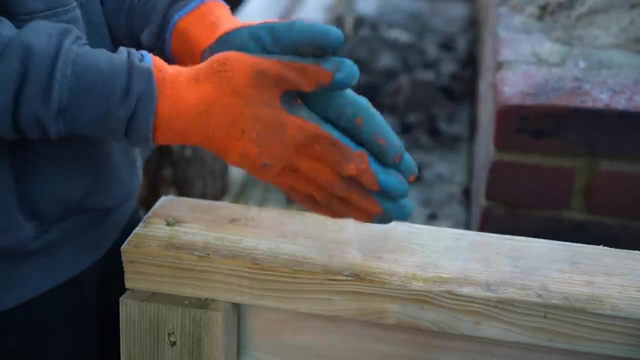 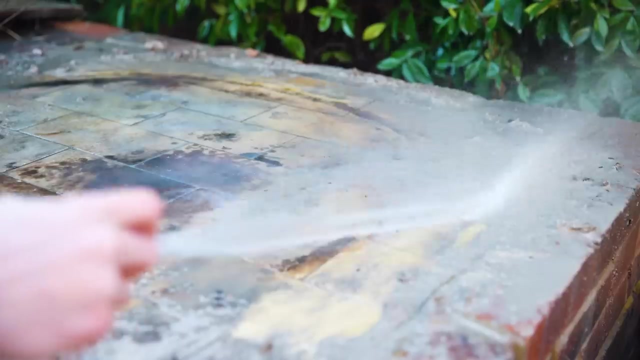 to get on with, and that was destroying the old pizza oven, removing it from the base so that it was ready to rebuild again. There we go: The old oven is gone, The base that it sits on is now clear, ready to be built on again. 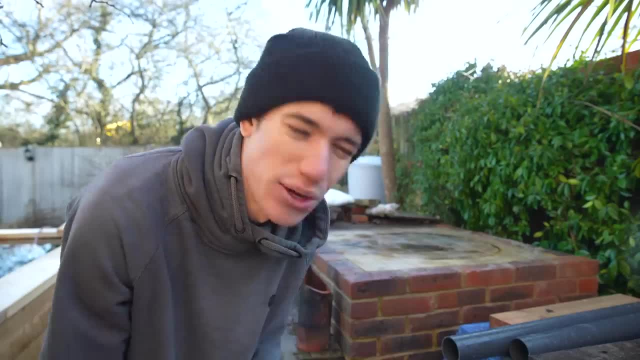 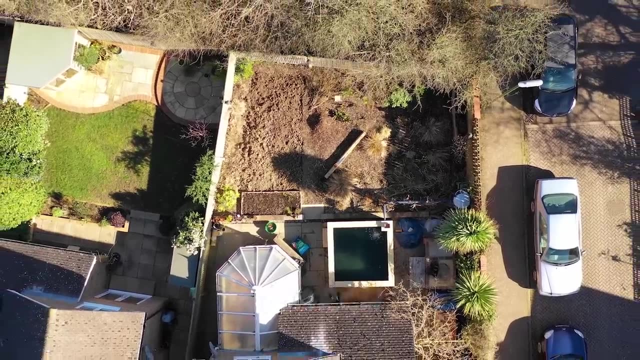 I've just got to have a think about how I'm going to do it this time, because I don't want it to break in the winter when it gets cold and wet. Finally, by the end of March, things were starting to warm up a little, Although the garden was still. 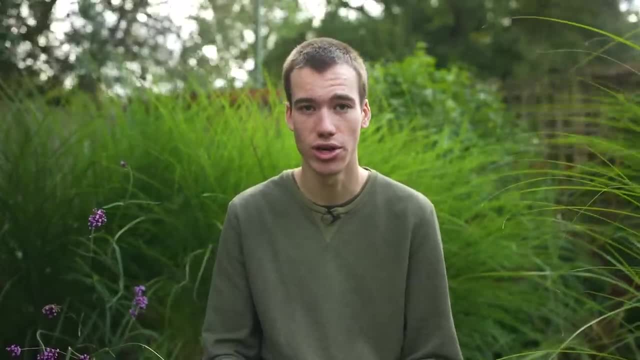 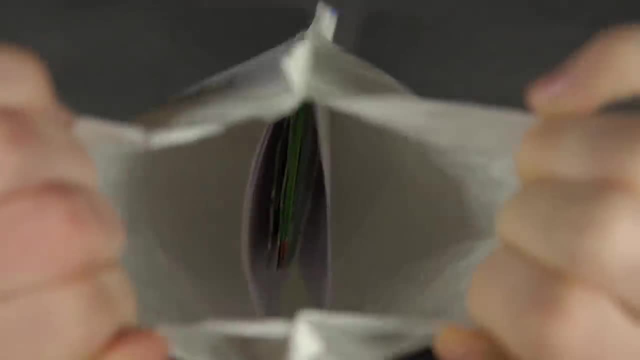 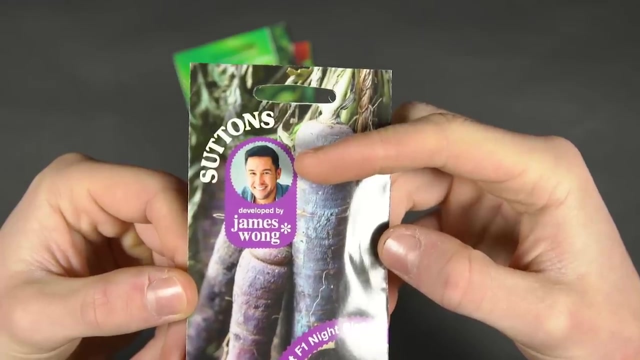 exciting. with that, I could start thinking about what I wanted to grow, And so I started ordering bulbs, seeds, and when I started receiving them in the post, yeah, that's when things got more exciting. I bought a selection of seeds, from carrots to cucumbers, even some of James Wong's. 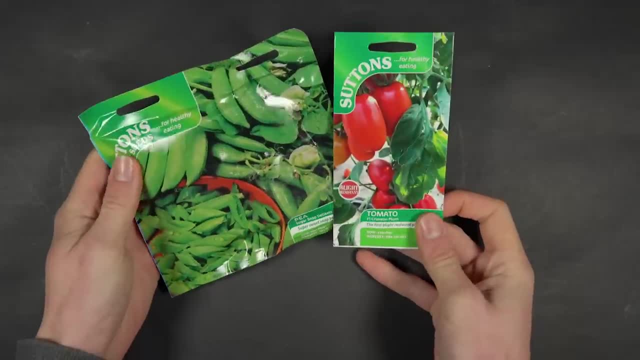 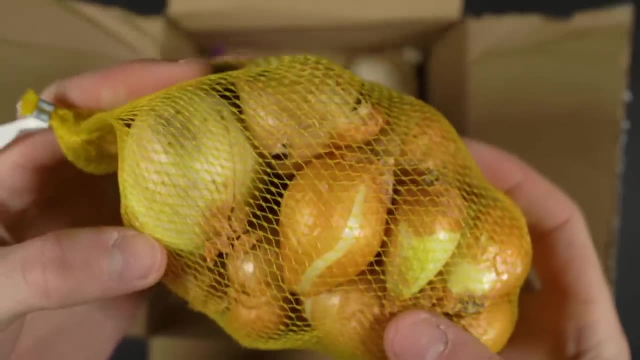 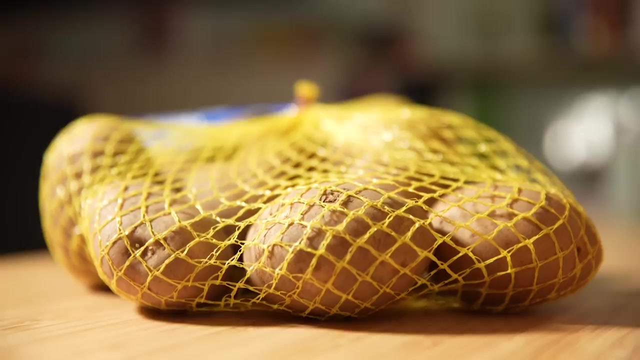 purple carrots. Also, I didn't forget my sugar snap peas and tomatoes. I also unboxed a load of garlic, shallots and onion sets and I was quite excited to get them in the post. I also had some seed potatoes arrive in the post And basically chitting is the process of. 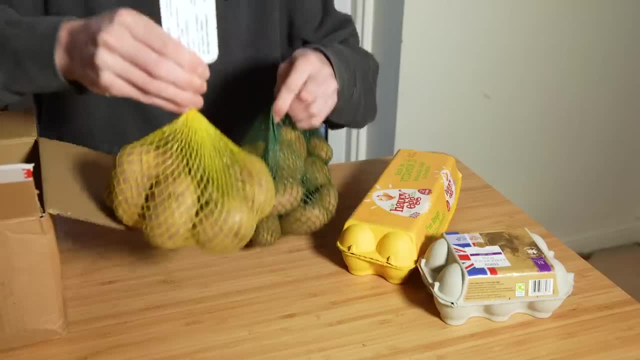 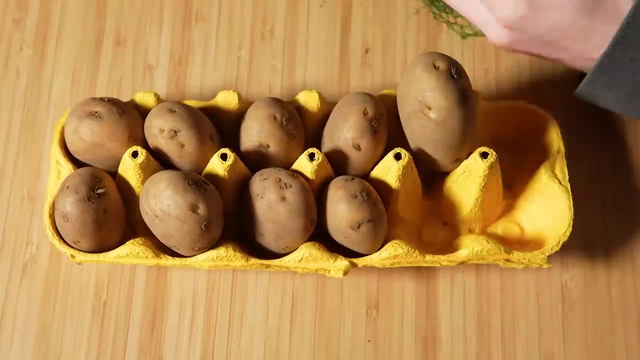 sprouting the potato indoors in like a warmer place and it gave them a chance to sprout. you know, get a head start And then when I put them in the ground they would be already ready and growing and then hopefully they would grow quite quickly. That's the theory anyway. That's. 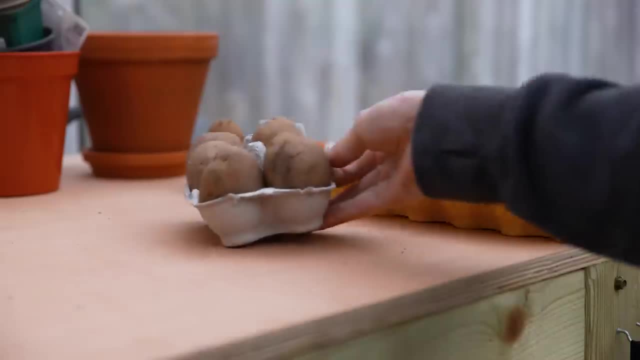 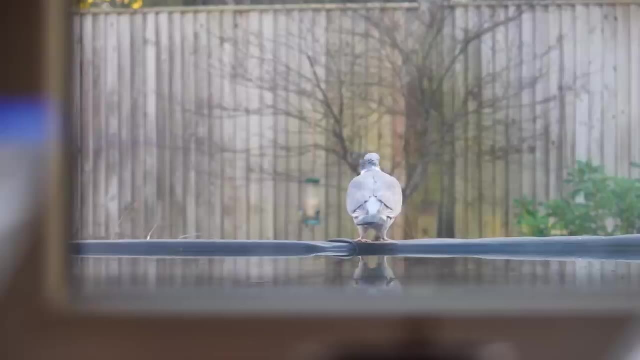 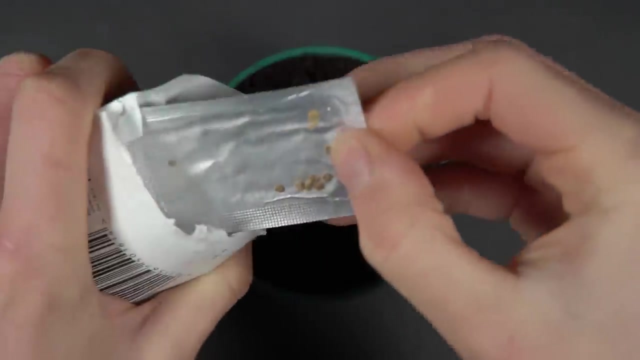 what I read in a book. So there are two varieties of potatoes prepared Over the next month. apparently they are. It's supposed to start to sprout and then they'll be ready to put in the garden. I also started germinating some seeds as well. I did some tomatoes, cucumbers. 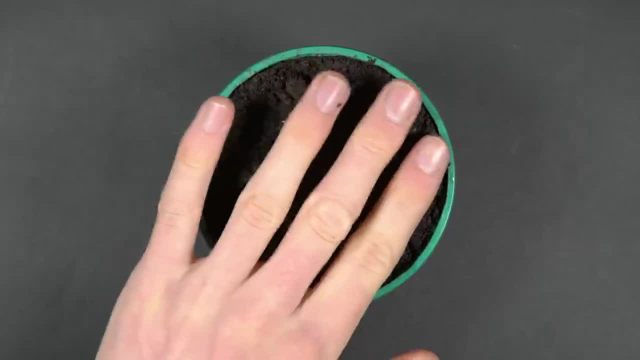 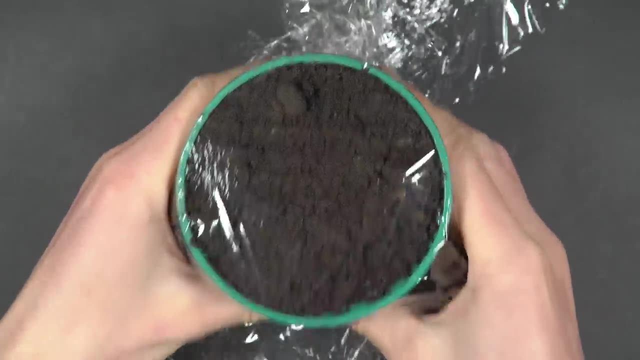 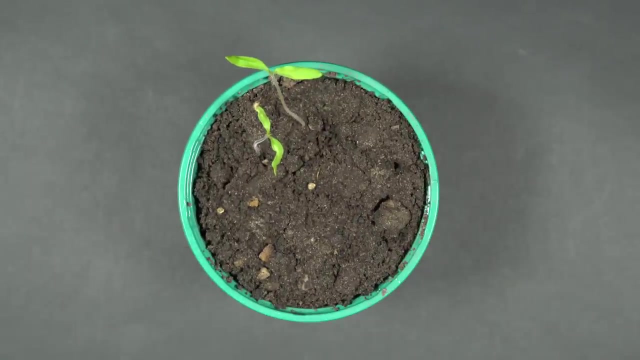 chilies, various other things as well. But yeah, the whole process of germinating is like super fascinating And it's just like a fun thing to do. You put a seed in some soil and then, over the course of a week or two, you watch it become another plant. It is like magic. 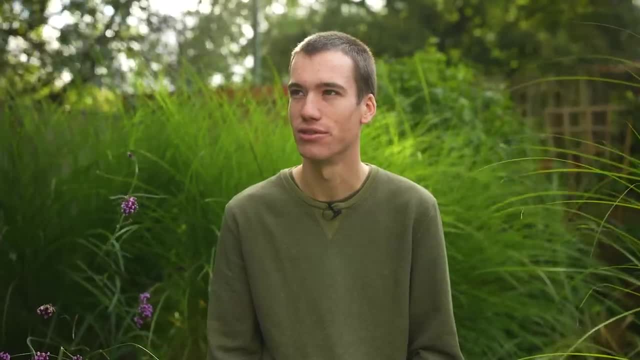 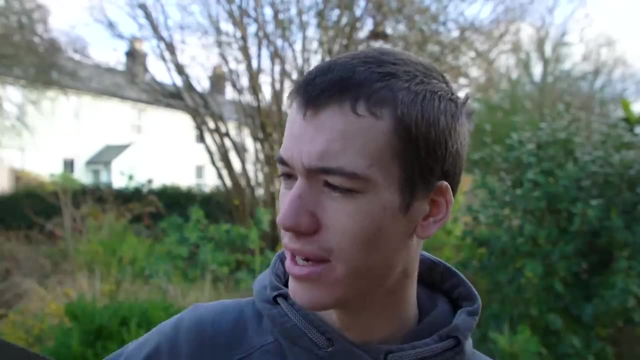 It sounds like that to me because I have no knowledge of how science works. I've got a saw, There's a hazel bush behind me and I'm going to get to work and cut off some branches to use as a trellis to grow peas up. 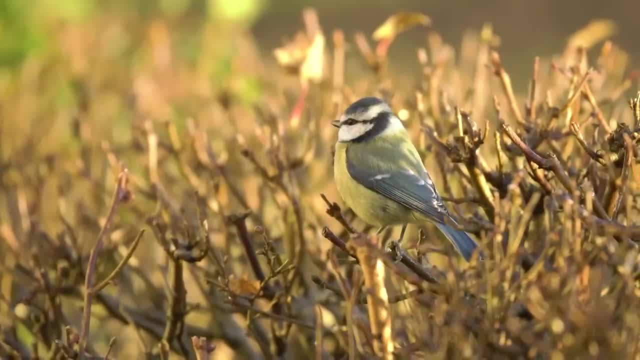 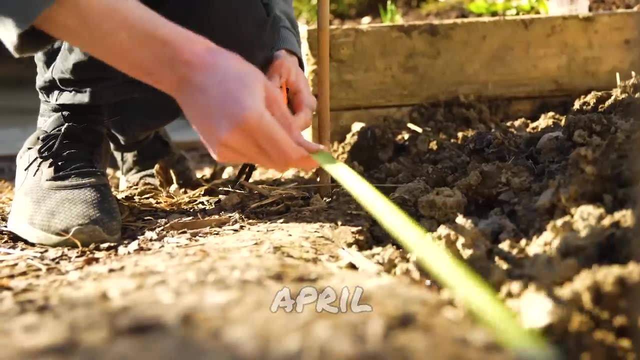 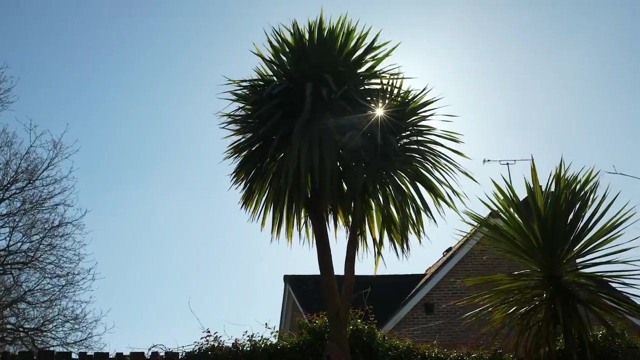 A few weeks later and spring was finally here, And because the ground had started drying out, I could start building My raised vegetable beds. Now, the reason for making raised beds, rather than just putting the vegetables straight in the ground, was that I wanted to add compost to the soil. The soil in my garden is so sticky. 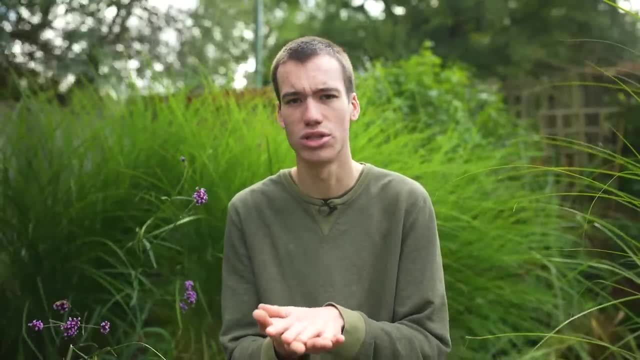 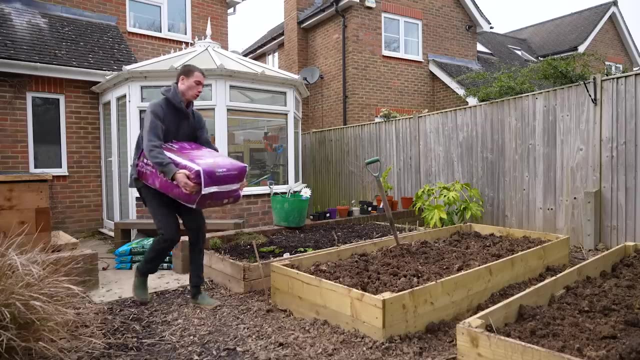 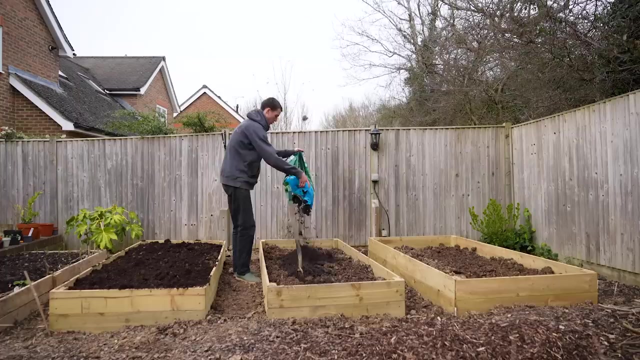 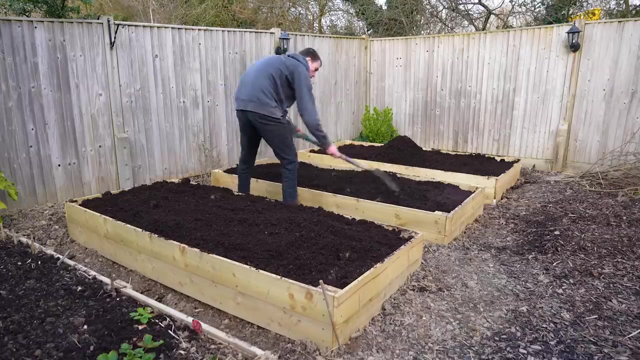 and compressed that water doesn't go through it. So my aim was to create these vegetable beds, fill them up with a mix of the clay and some compost that would loosen the soil and create a better growing medium for the plants. Until quite recently, I very ignorantly thought that soil was just dirt. It was. 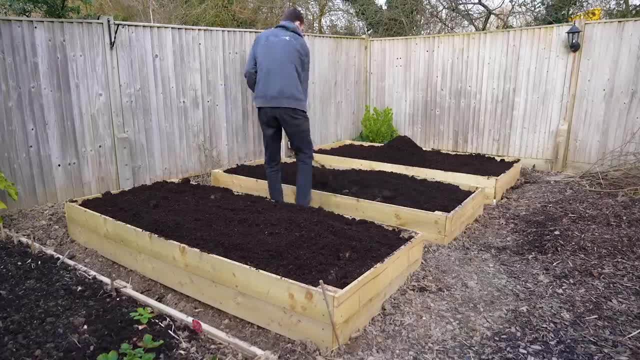 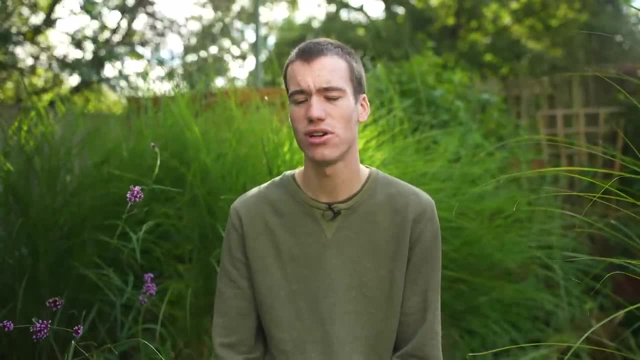 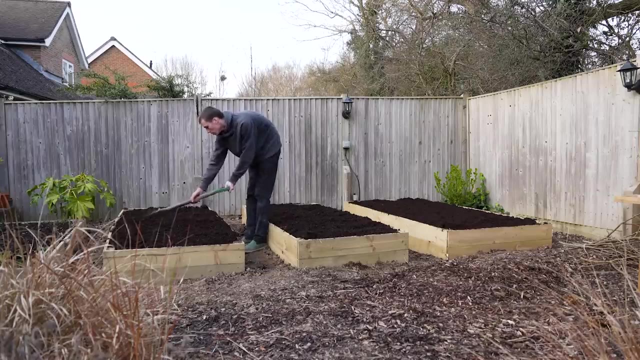 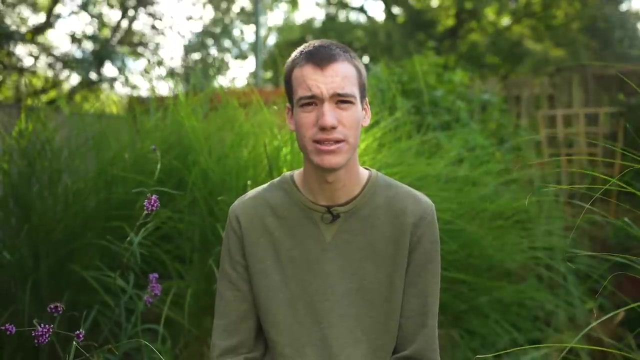 just this brown stuff on the ground which had no real purpose, and it was annoying when it got on your clothes and made them all dirty. But how wrong I was. Soil is, firstly, incredibly complex and, secondly, it's incredibly important for life. It's a mix of minerals, nutrients, bacteria, fungi, animals like worms, millipedes. 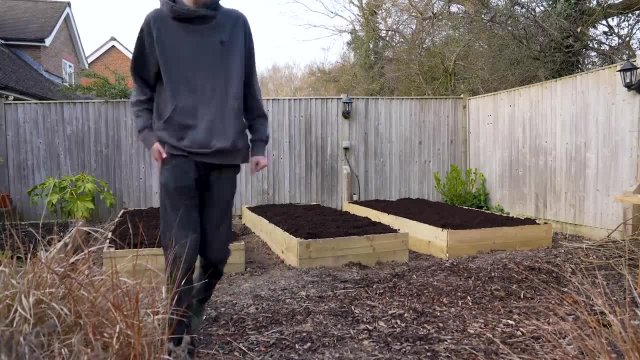 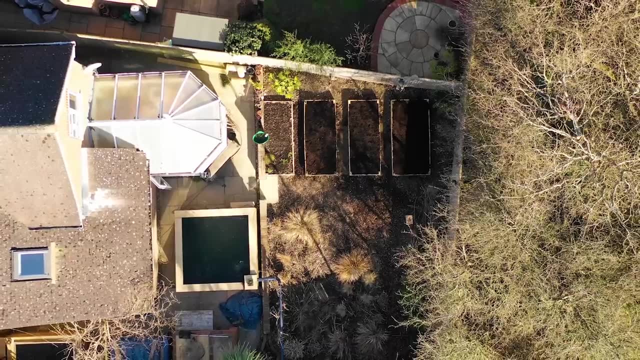 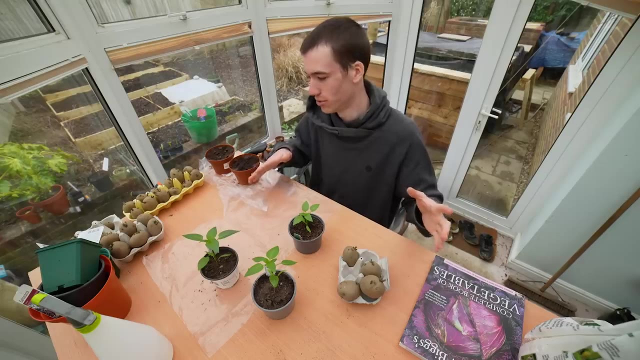 Basically, what I'm saying is: it is a living thing, It is very important, and you need your soil to be good quality if you're going to be able to grow vegetables and have food to eat. Finally, it is time to start growing some vegetables. In fact, I've already started. 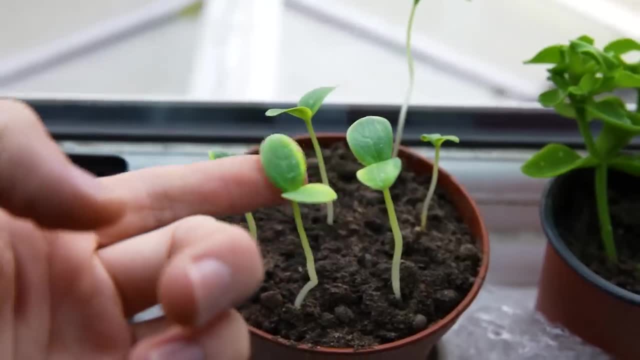 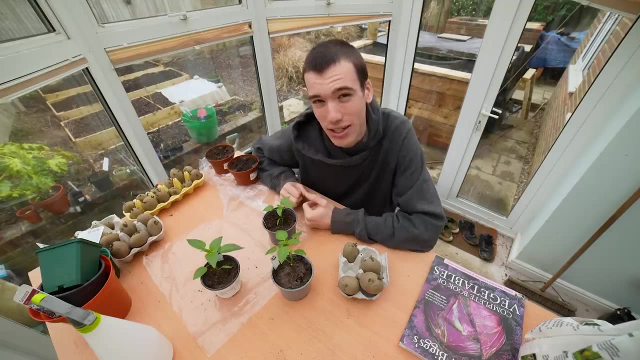 I have been very eager to get going and start planting a few bits, and I think I'm going to do some carrots today, and then I've also got some onions, some garlic, some shallots, So I've got plenty of stuff to get going, and also those potatoes that I prepared has actually started. 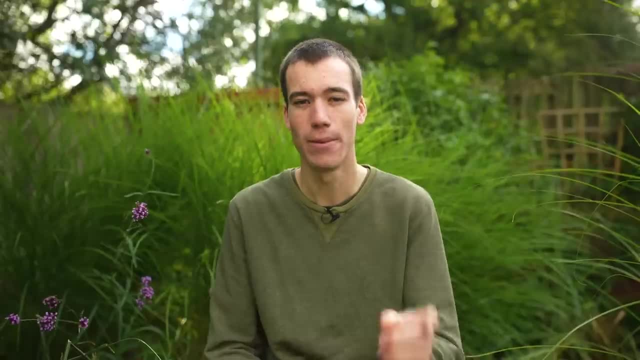 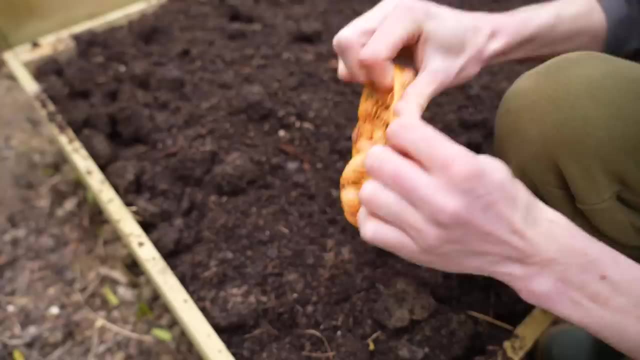 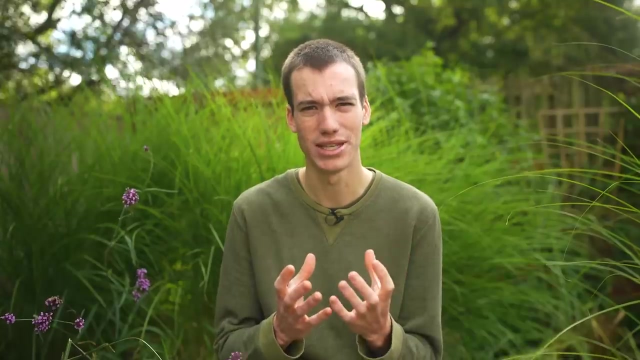 sprouting, so they would be ready to plant very soon. But the first thing I actually put in the ground were onions, and I bought these as sets. Now, sets are basically just like baby onions that you put in the ground. Over the course of the year, hopefully, they expand into great big bulbous beauties that you can put in. 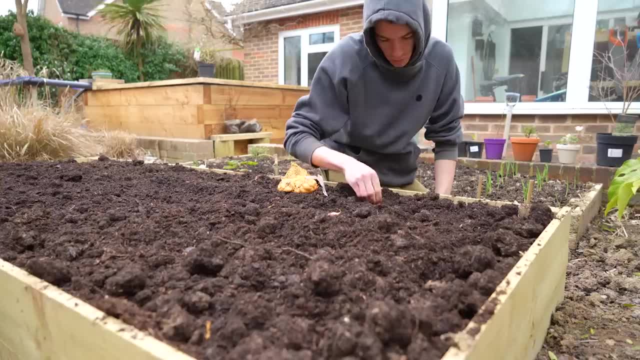 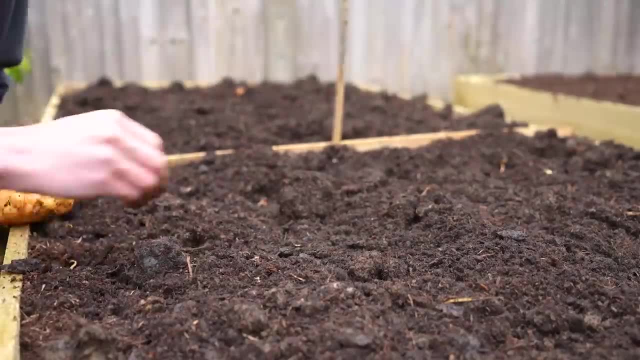 your bolognese. So I put them in the ground just with the tips just poking out. That's how your men apparently do it- And, yeah, basically just left them. I think I planted 60 or 70 of those. So if 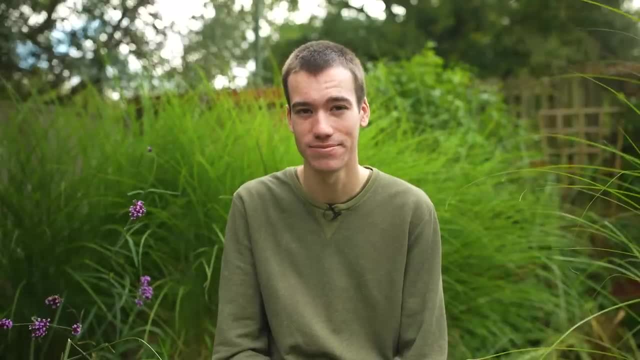 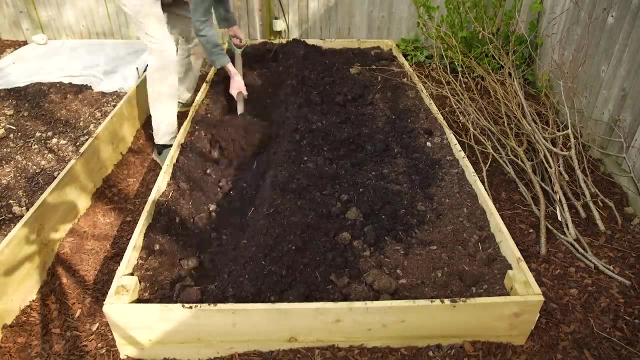 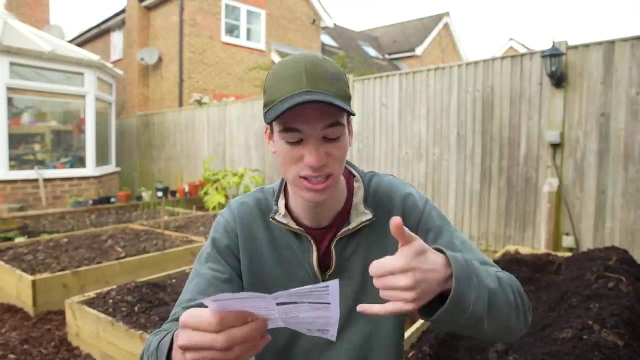 they all were to turn into big onions, it was going to be a pretty good harvest. Today is actually going to be the first time of my life where I've tried planting potatoes, So please bear with me if I'm doing everything wrong. Four inches deep, 30 centimetres apart, 45 centimetres between rows. Let's get planting then. 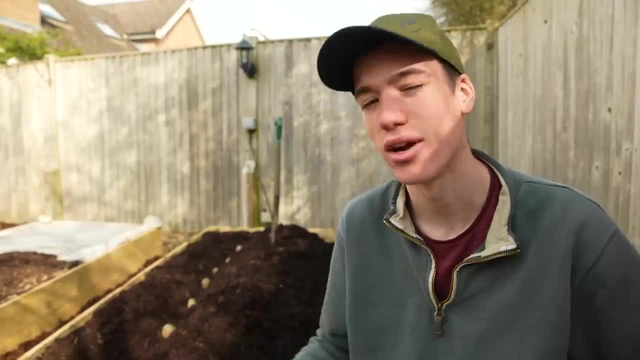 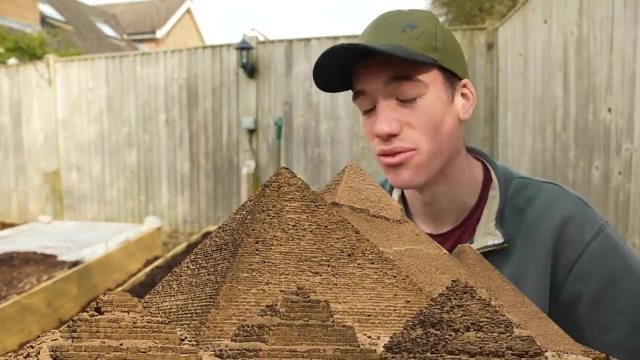 One of my fondest memories as a kid was when we were driving back from holiday. I think it was in Somerset. In the distance I saw what looked like a pyramid and as we got closer I realised it was no pyramid, It was a mountain. 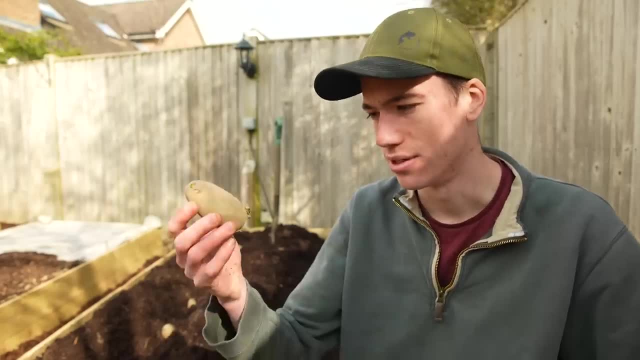 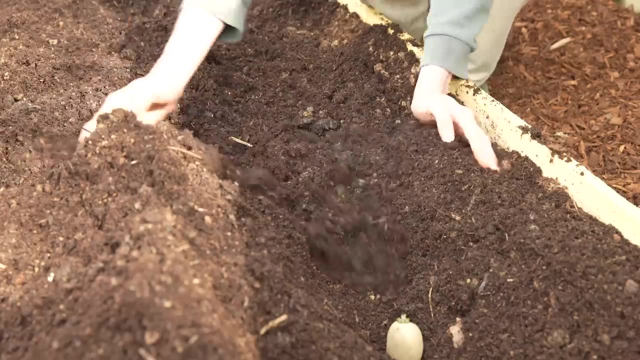 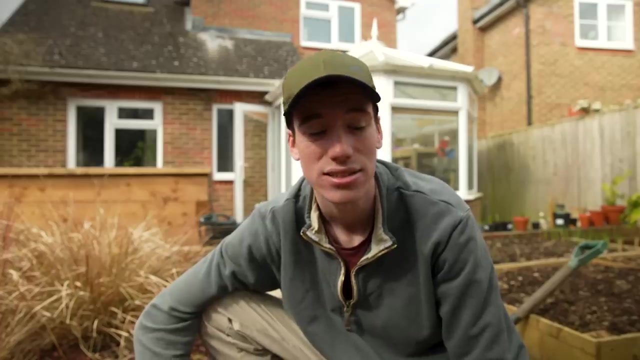 A mountain of potatoes. I'm going to shut up and plant some more potatoes And there we have it: The potatoes are in the ground. I think they take around 100 days, So I've just got to be patient. But I'm looking forward to it because 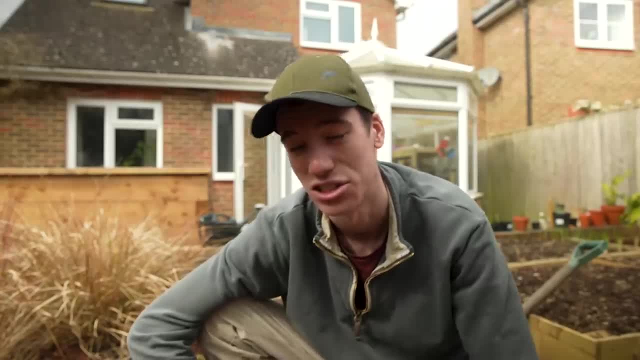 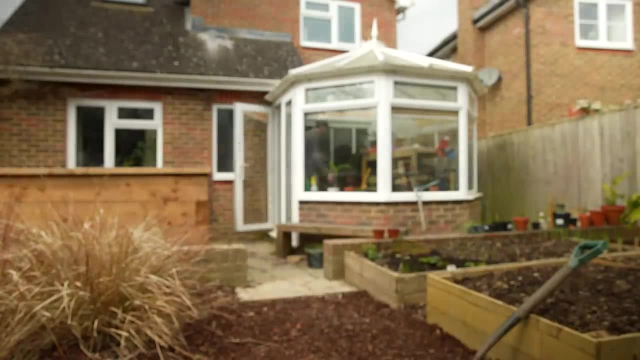 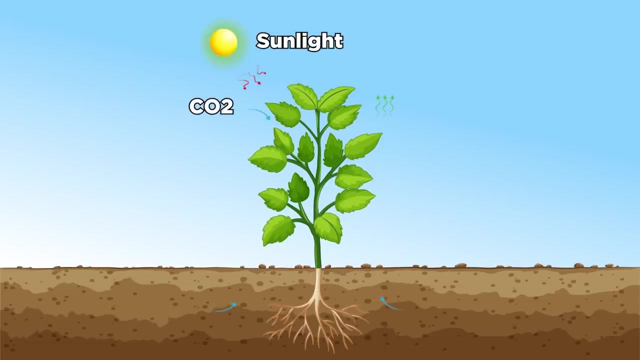 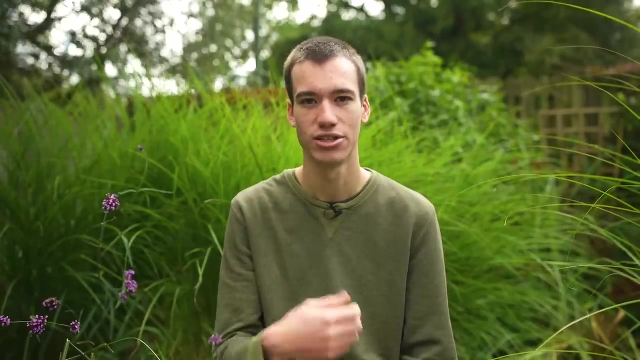 I absolutely love thick cut fried chips or roast potatoes on a Sunday afternoon With plenty of stuff in the ground. I then patiently waited. Now plants grow by photosynthesis using sunlight and CO2 carbon dioxide from the air and convert that into sugars which they use as energy to grow. 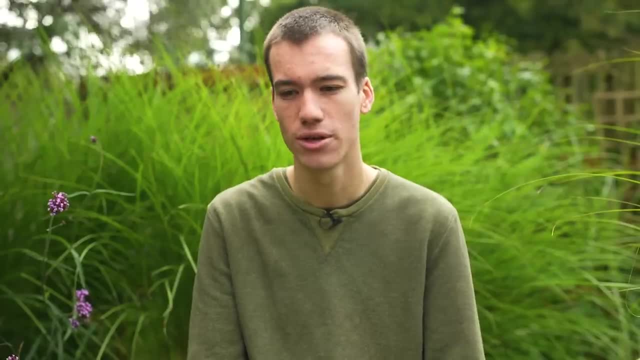 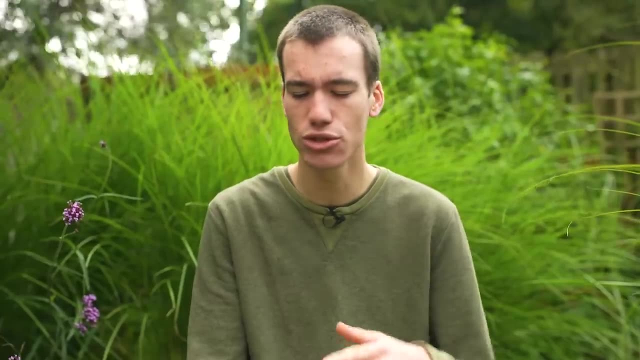 They also take up nutrients from the ground through their roots. I think the main ones that gardeners talk about are nitrogen, phosphorus and potassium. There's also a tonne of other things that plants need, But yeah, those things are necessary for plants to thrive. 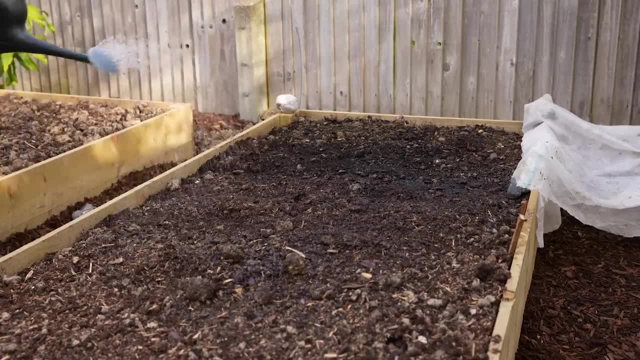 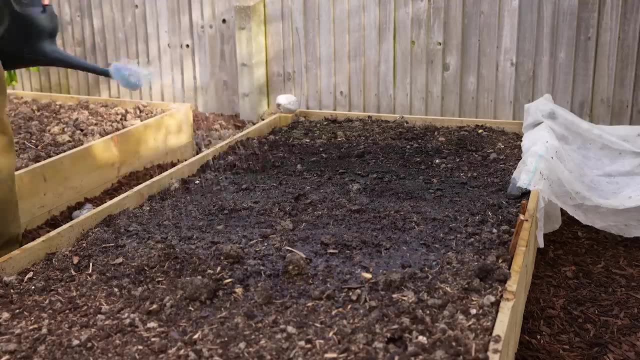 And so I hope that my soil would be good enough. The only thing I really had to do regularly was water the plants, So at most mornings I would put my finger down into the soil, check whether it was dry or not, and then water if necessary. 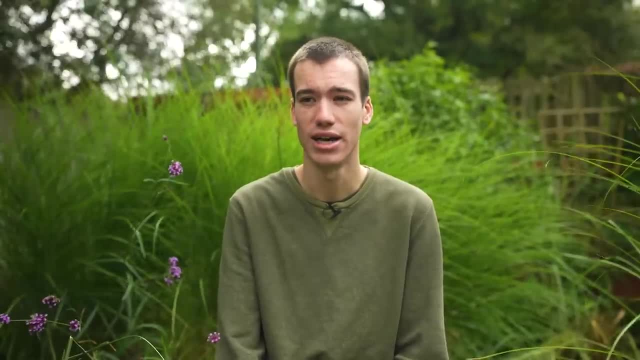 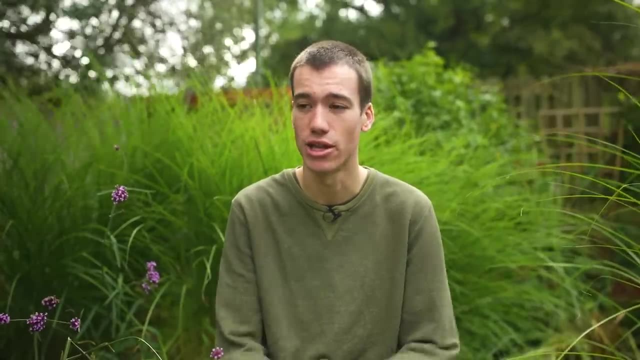 And throughout parts of the spring we had some proper dry, hot weather and I had to water it like twice a day and keep on top of that, I lost a number of spring onions because I just forgot to water one day and they all just frizzled up and died. 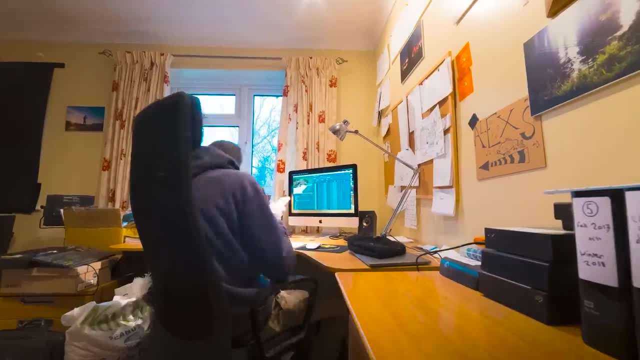 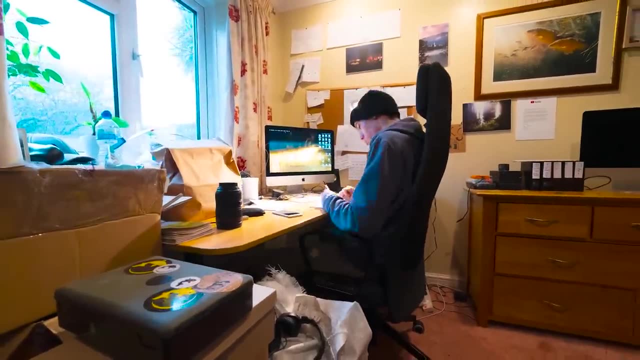 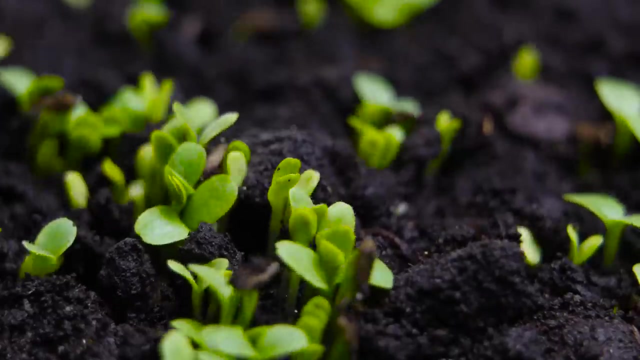 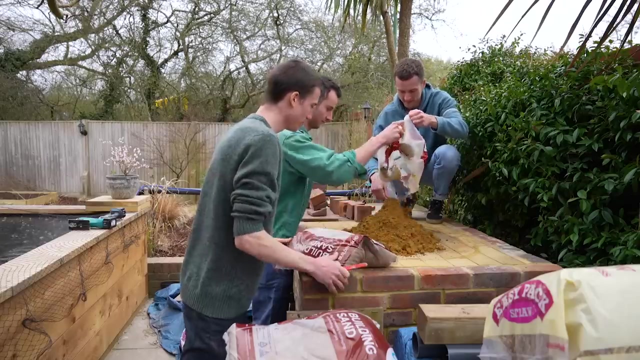 But other than that, I pretty much just waited, got on with my life and waited patiently Whilst I let the plants grow, I found the time to rebuild the pizza oven, and a couple of friends helped me out with this. Firstly, we made a large mound of sand. 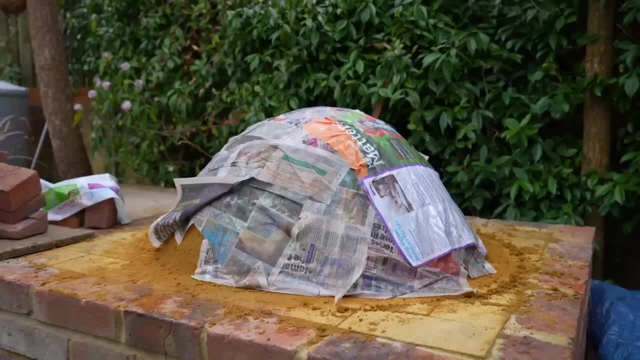 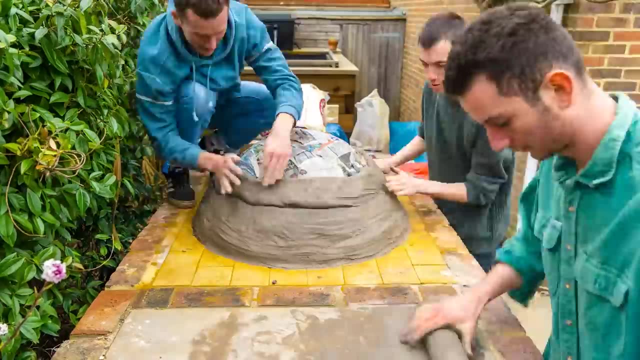 This would create the oven space inside. Over this we lay some sheets of newtonite, and then we used newspaper to stop the clay from sticking to the sand, And then we finally built up a number of layers of clay. For the entrance to the oven we built a brick arch. 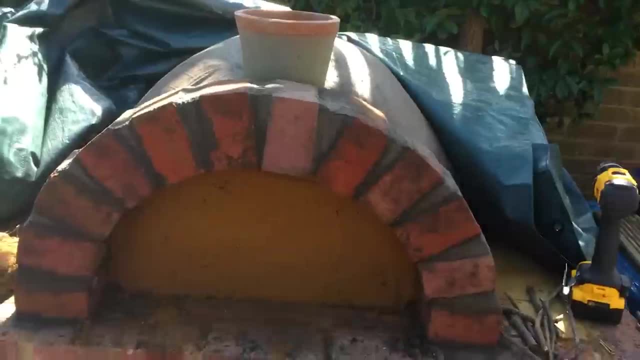 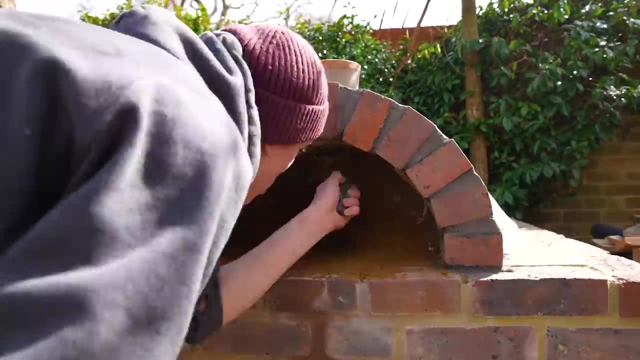 which I quite like the look of. The wooden former was removed and I put on another couple of layers of clay. I could then scrape away all the sand from the inside of the oven, which reveals the newspaper that I used. That will quickly burn away once the oven is lit. 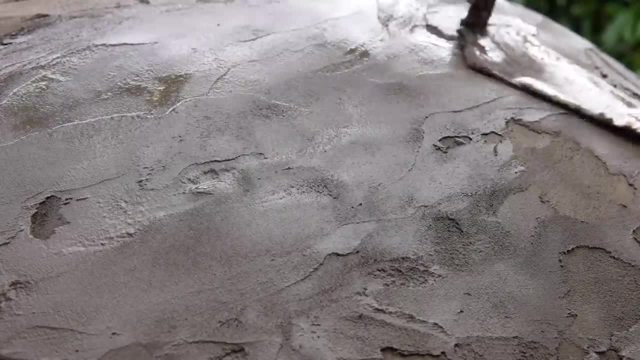 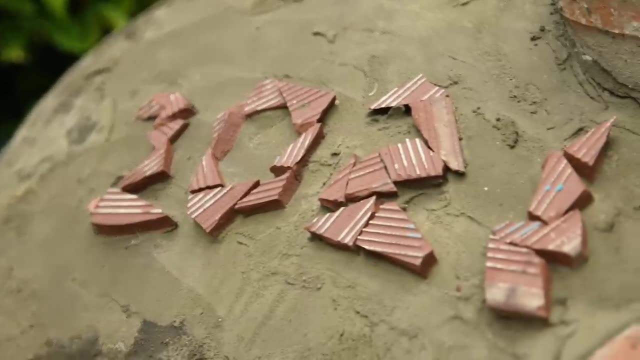 A final layer of outdoor cement was added to make sure it was waterproof. It was good to finally get that project out of the way, and hopefully it would last a little longer than last year's one, As well as my 15 square meter patch in the garden. 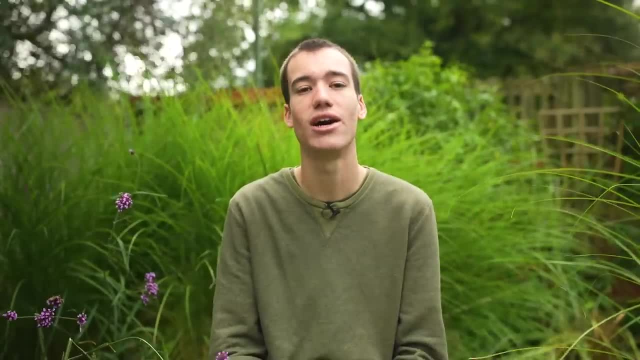 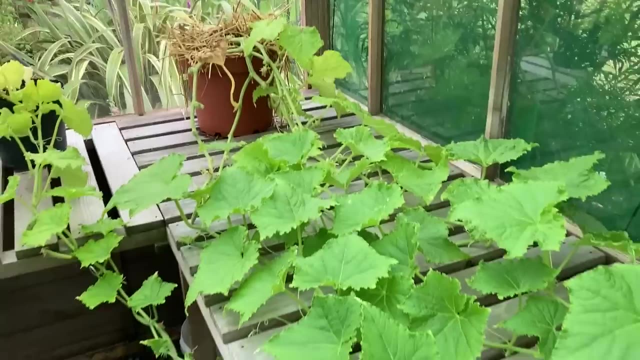 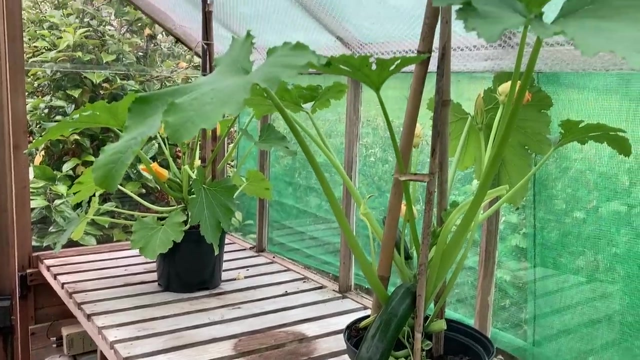 my dad, who lives 15 minutes down the road, very kindly let me use his greenhouse to grow some other stuff. I've got two cucumber plants which have just decided to go crazy and spread all over the place. Then I've got a couple of courgette plants as well, which are looking good. 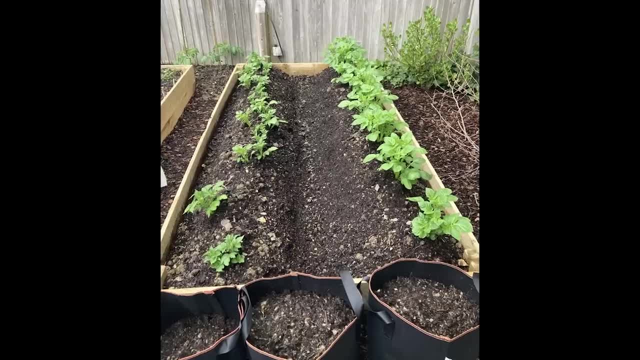 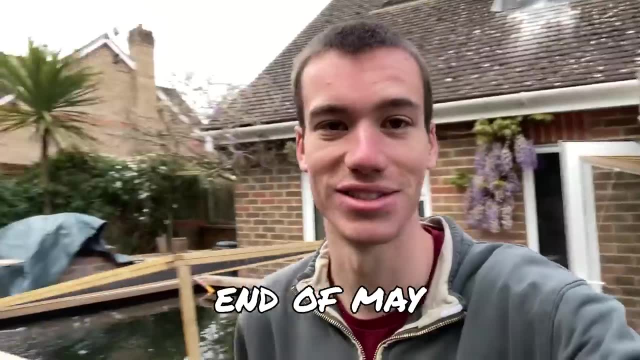 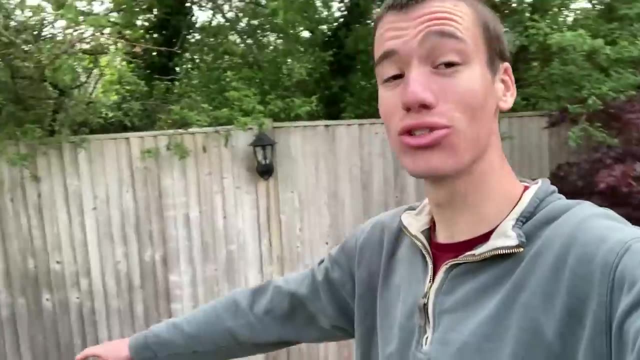 Yeah, Thanks, dad. Let me use this little space. Quick update on the garden. Everything is growing so much. When you last saw it, these were all pretty much bare. Check out the potatoes. They have grown so much. Look at that. 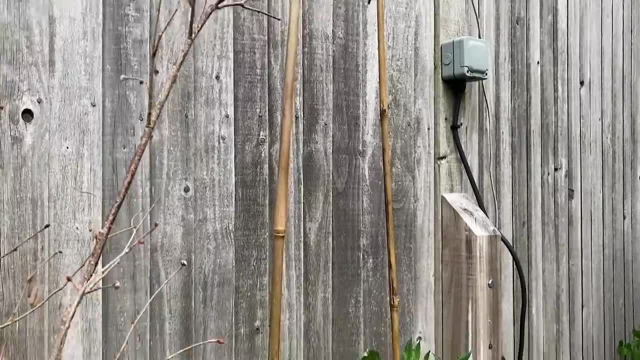 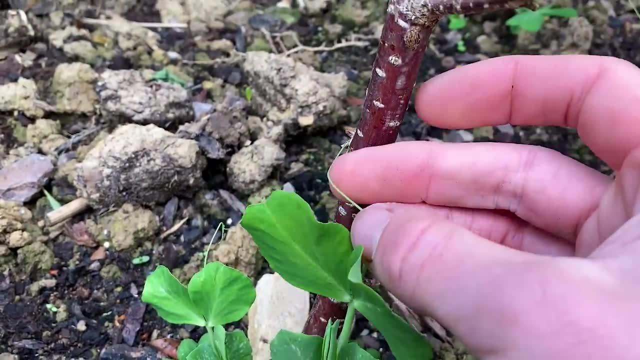 I've got two different varieties of potatoes and I've got some tomatoes over there. Check out these. This is so cool. So these are sugar snap peas. They grow like these whiskers and they use them to attach themselves to the thing that they're climbing up. 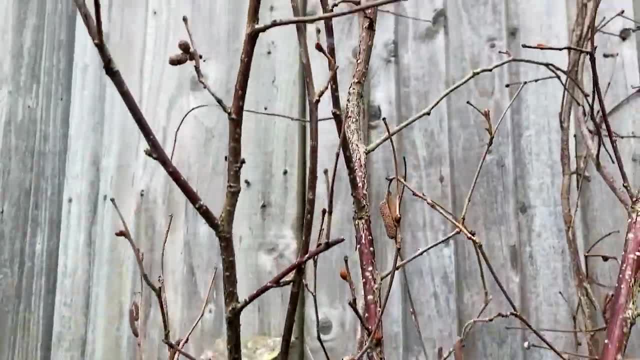 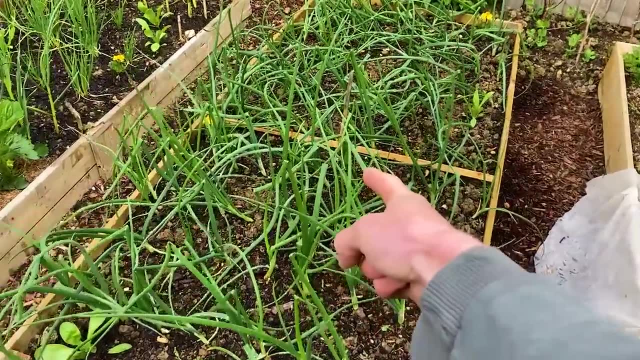 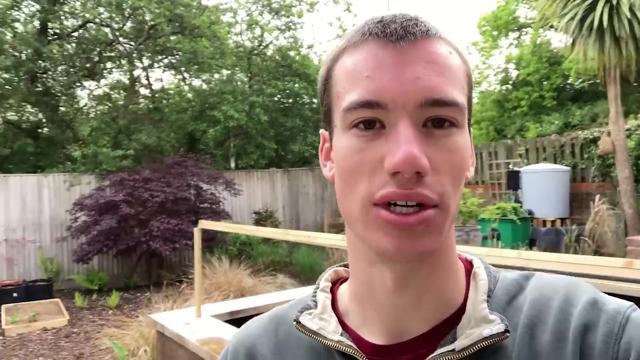 so they can go right to the top. And I've got loads of carrots that I've been growing from seed, onions, garlic, even some strawberry plants, some courgette plants. The list goes on and on and on. We're going to have so much food later on this year if it doesn't all die. Fingers crossed. Fast forward to the 3rd of July- I think it was 100 days after I planted the potatoes and I decided to have a little look and see if they were ready to harvest. Hey guys, let's see what we've got. 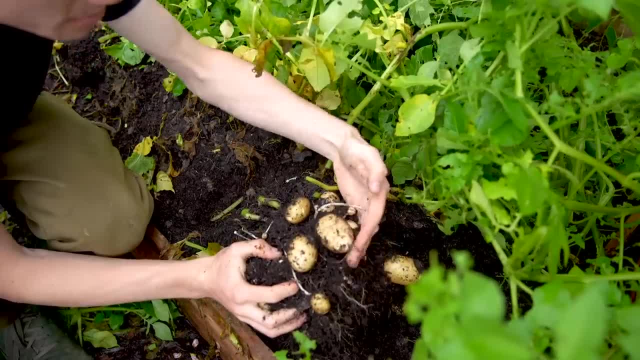 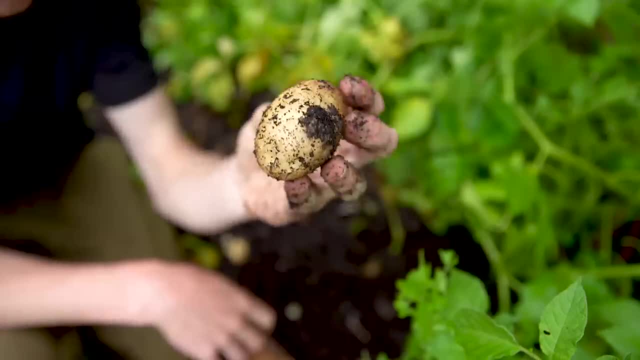 Oh, no way, That's way better than I thought. I had Whoa Lots of small ones as well. Oh, that's a beast. Wow, it's going straight in my basket. That there is the potato which I planted, the seed potato. 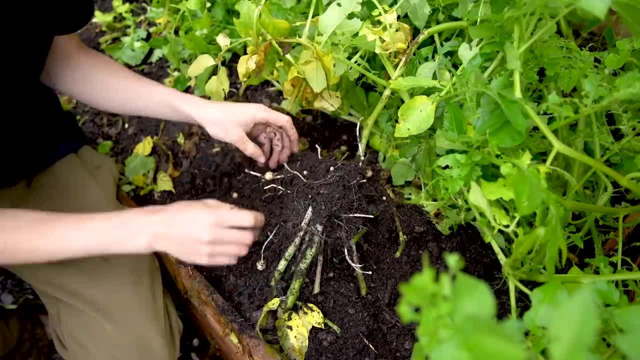 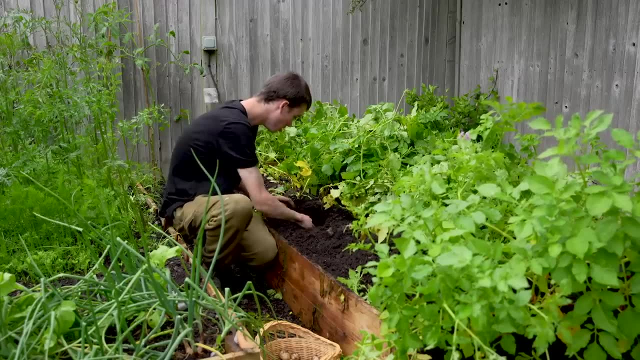 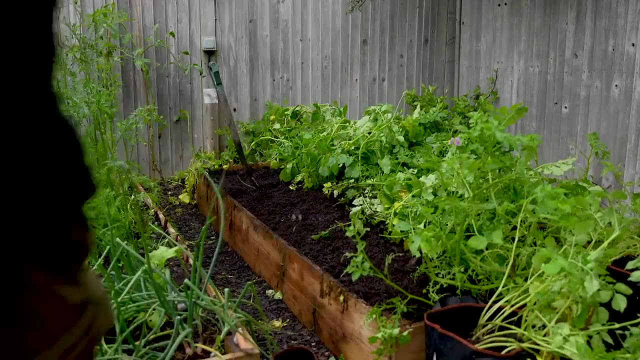 Ended up with all these other ones. This is fun. This is like digging up treasure. I was quite impressed with the result. I managed to fill a nice little basket full. I know it could have been better. I would have preferred if all of them were a bit bigger. 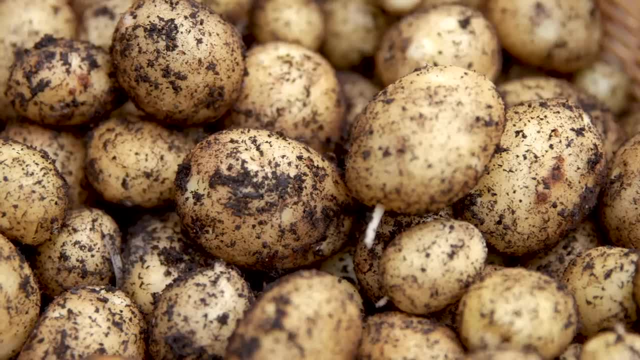 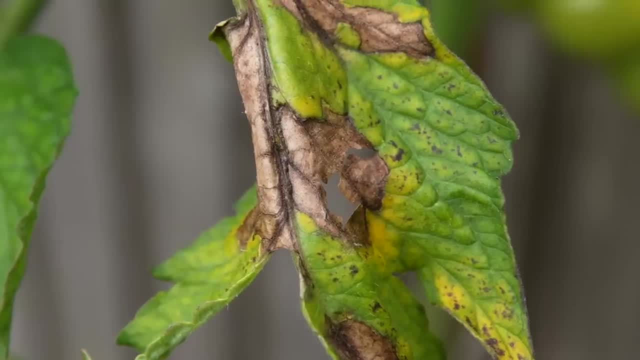 But you know, first time, first crop of potatoes. I was quite happy And I still had one more row that I was going to harvest a bit later on in the year. However, not everything in the garden was flourishing And for reasons I just didn't have a clue. 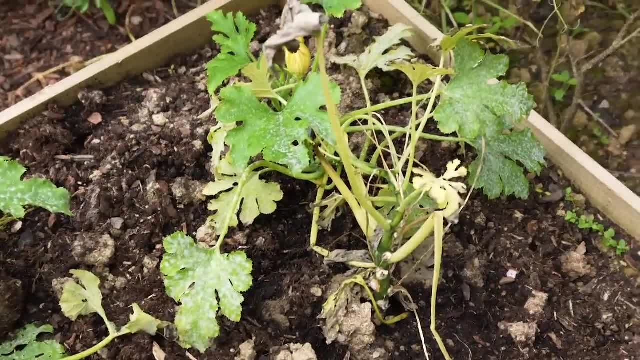 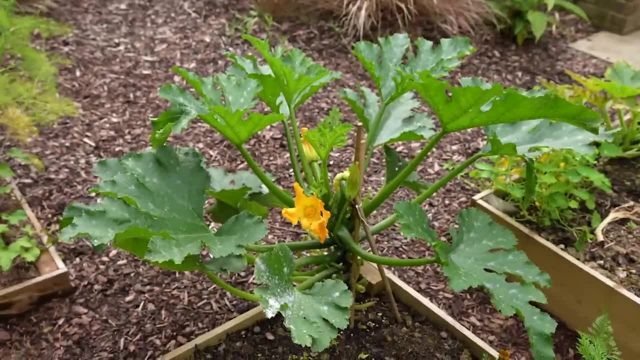 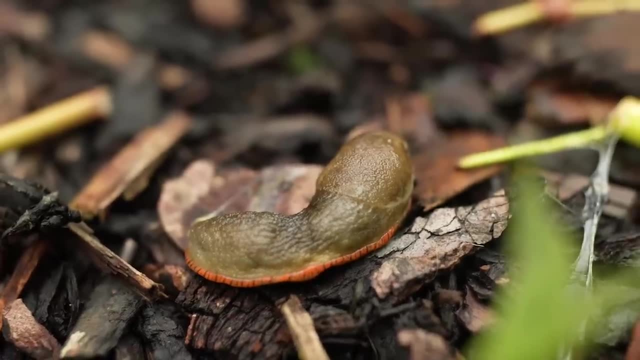 Well, these courgette plants just don't look very happy, And I don't have a clue why This one, however, look at that, It's a beast. The biggest pest we have in this garden are slugs. Now, I'm not going to lie: they are my least favourite living organism on Earth. 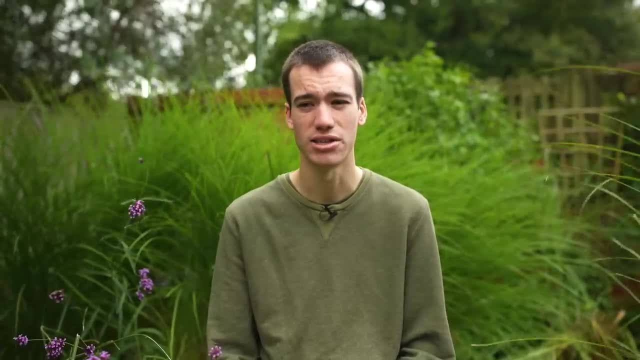 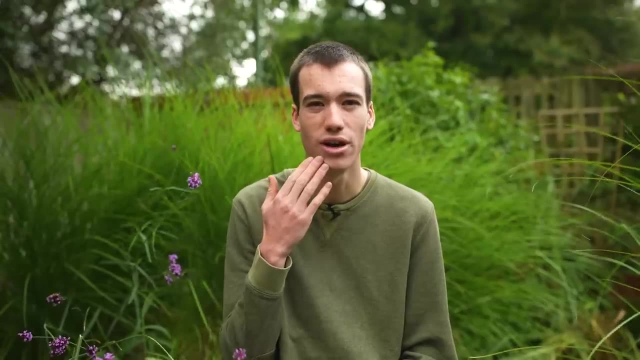 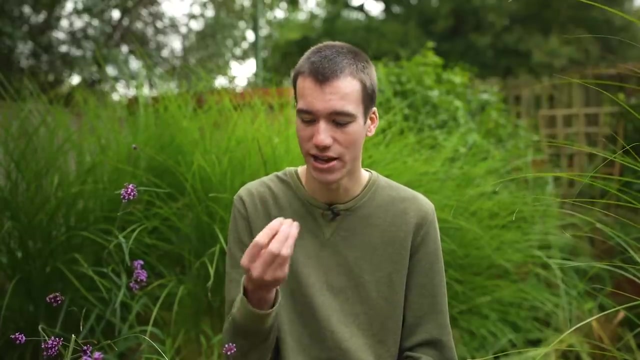 It's probably because I've had a bad experience with slugs in the past. I was out camping one night And a slug had crawled up my body, over my mouth, And I woke up to a slug on my mouth. I pulled it away and it like peeled off and it left like a layer of slime on my face. 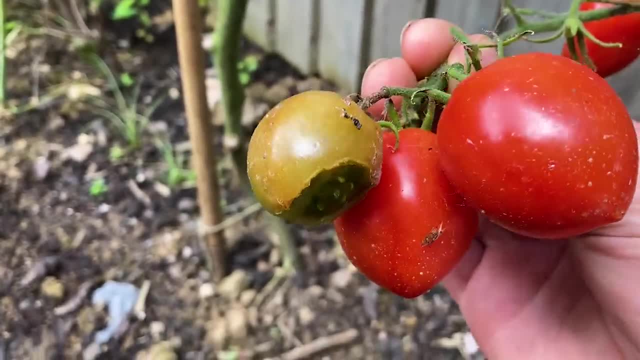 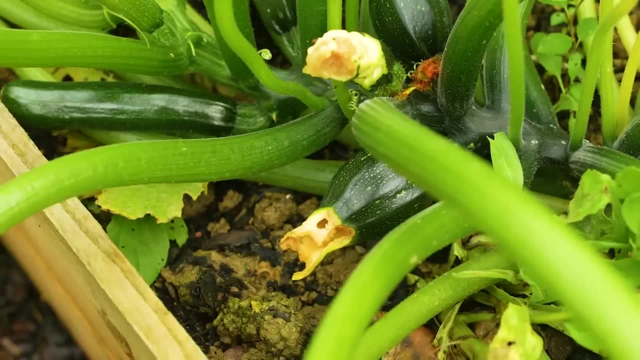 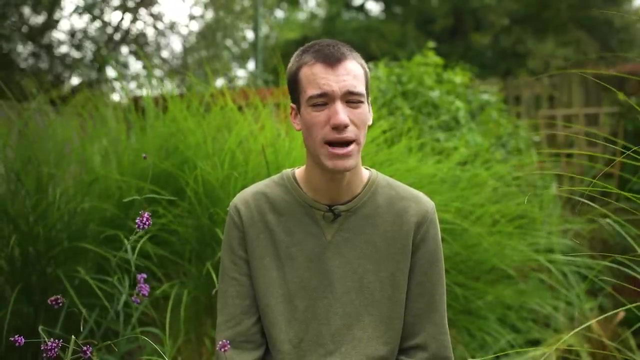 What is that? My tomatoes are being eaten. Oh, they just keep eating the courgettes as well. Maybe I need to get chickens. Chickens eat slugs as well. That might be the way forward. But yeah, slugs are a right pain. 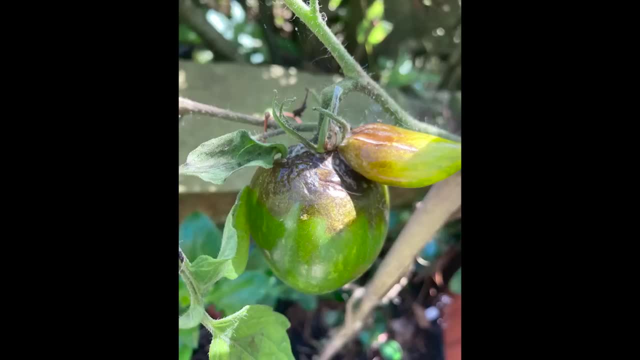 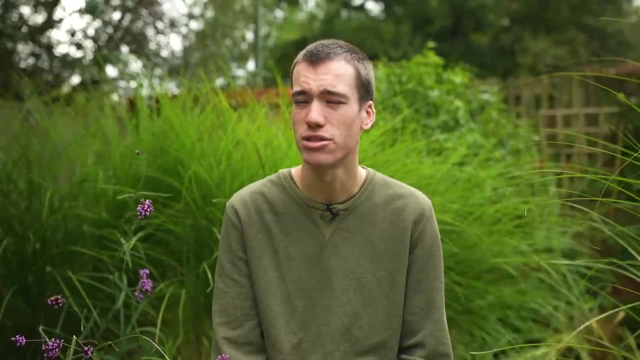 I also had some sort of disease on my tomatoes. I think it was blight, because one of the plants just went really black and everything died. Still, though, a couple of tomatoes managed to survive, and I managed to get them a bit later on in the year. 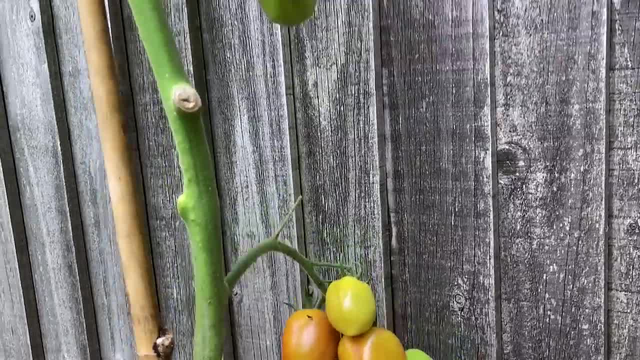 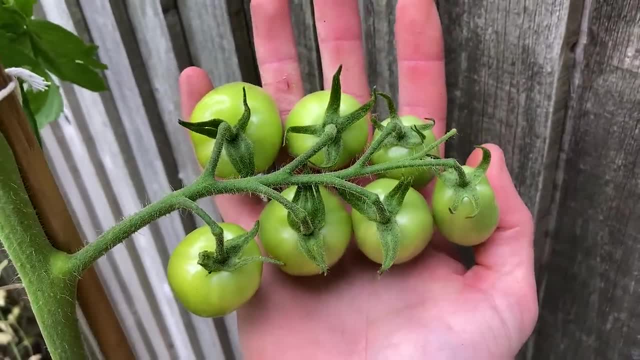 These ones are starting to go red, And then the further we go on, the better they get. actually, Look at that, there's a full set. Every single flower produced a tomato, But other than the diseases and the slugs, and what have you? 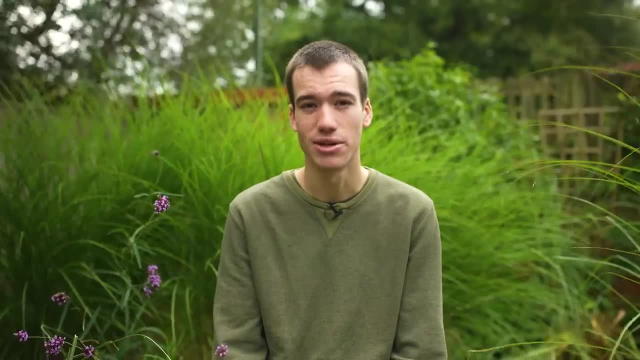 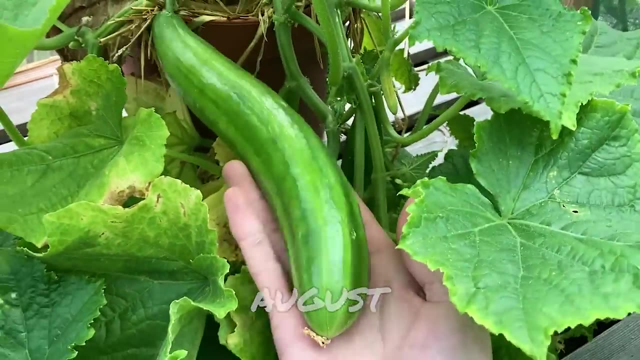 things started to get really hectic late in the summer and the harvests were coming in thick and fast. Well, that has to be my biggest cucumber yet. Look at that, Oh nice. Oh, there's some baby birds stuck in the greenhouse. 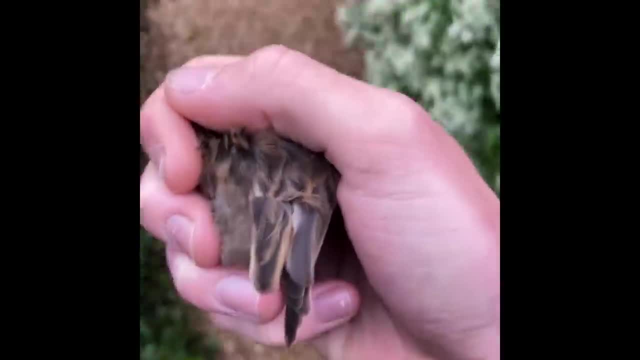 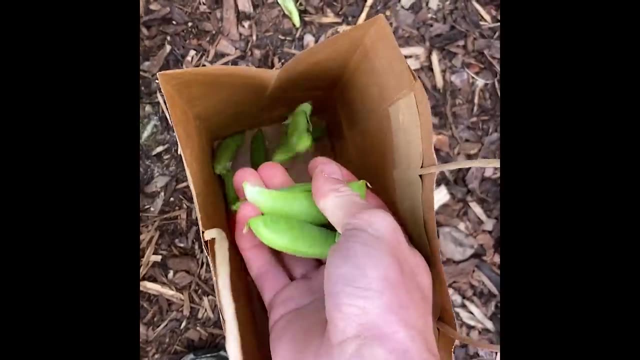 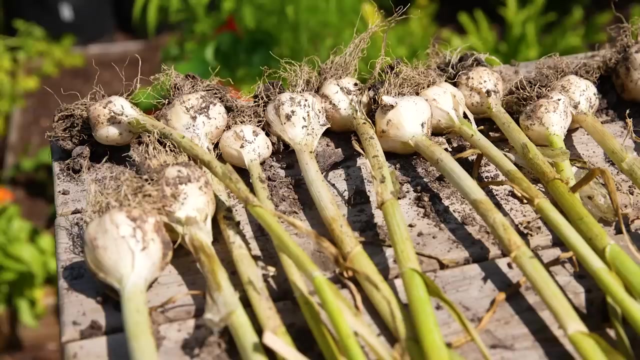 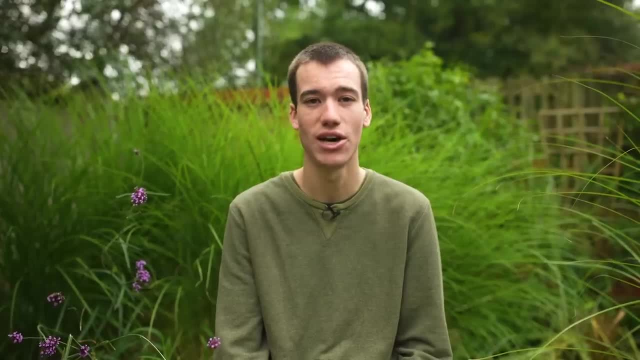 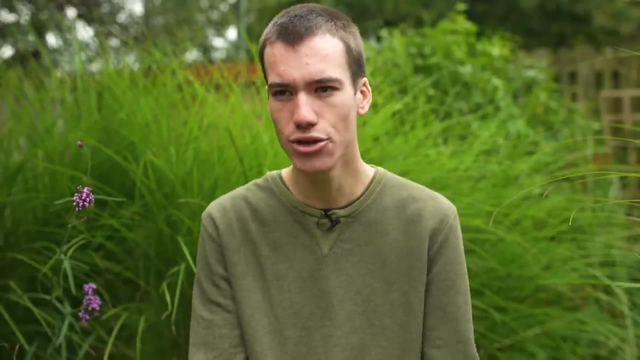 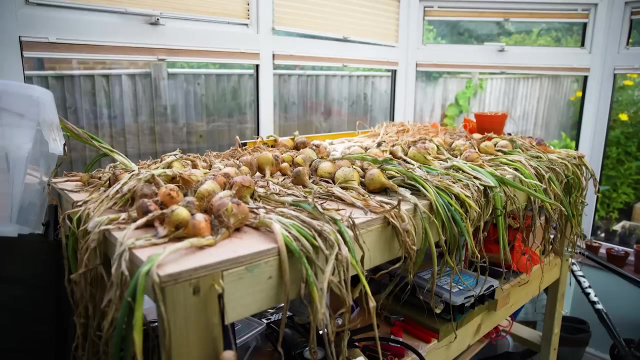 The crop was massive and there was probably going to be enough to last me throughout the whole winter, So I needed to prepare these onions so that they lasted me a long time. And you do this through a process called curing, And it's basically by drying out the outside layers of the onions. 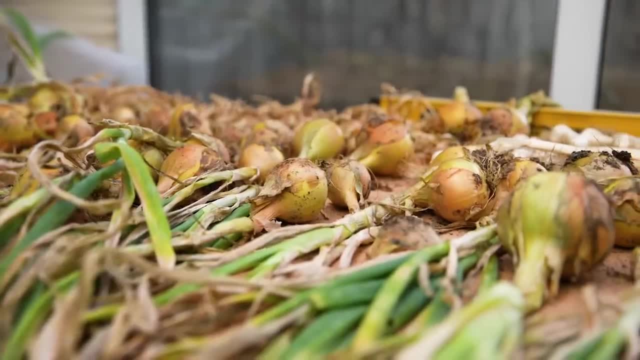 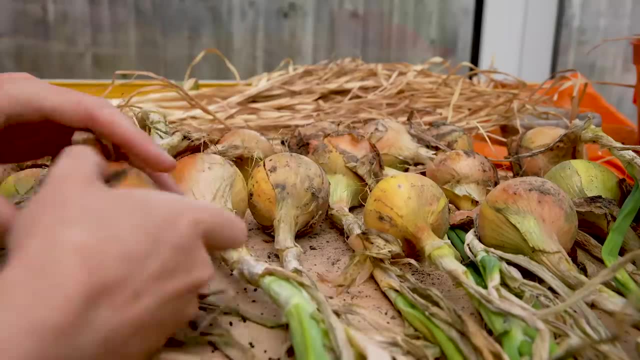 it protects the inner capsule and makes them last a lot longer. So I put them out in the sun for a few days and then left them in the conservatory for probably four weeks And the whole outside layer dried out. They were ready to store. 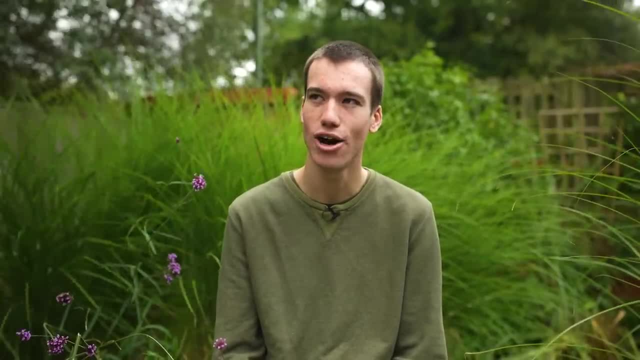 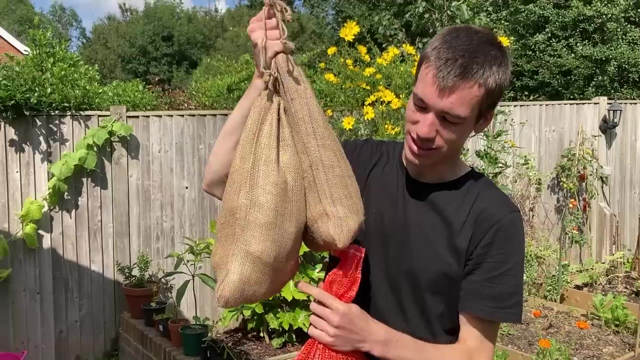 I put them into sacks. And yeah, holding a sack of my own homegrown onions was a very good feeling, I have to say, So it was a good day of harvesting. today I've got a couple of Hessian sacks full of potatoes. 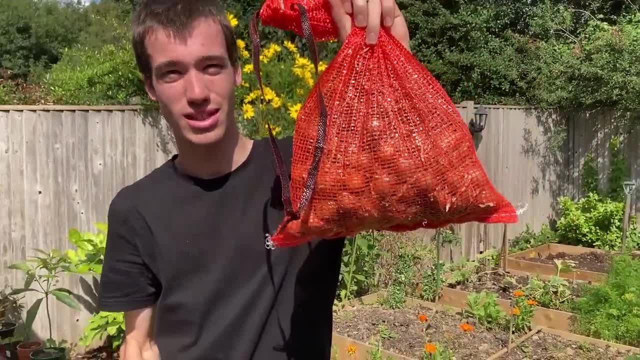 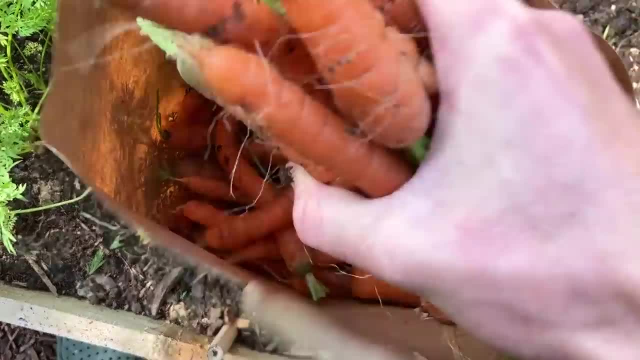 and also half-filled. I've filled this bag with some shallots And we've still got quite a lot to go, so things are looking quite good And by this point in the season I was actually regularly getting enough food to not have to get any vegetables from the supermarket. 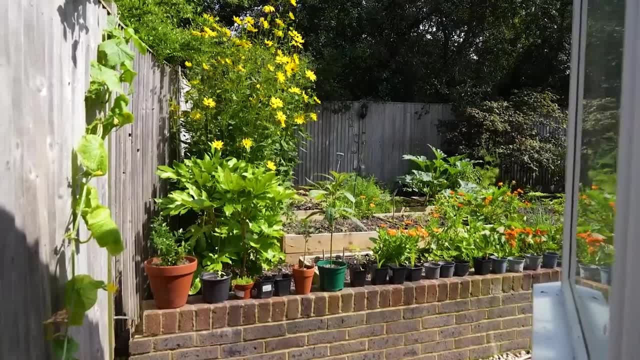 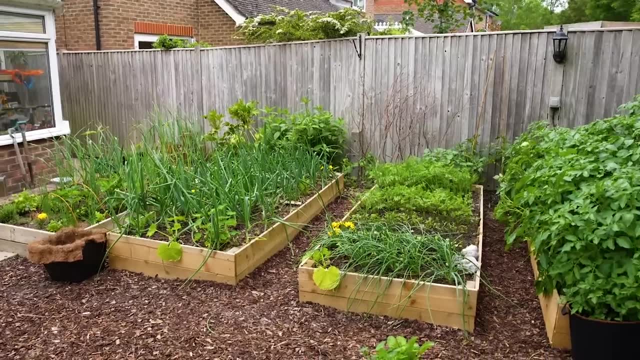 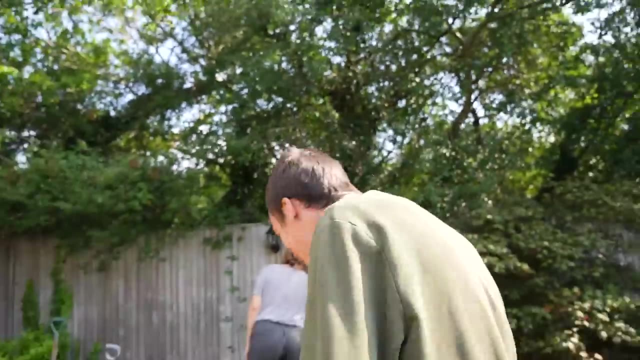 I had garlic, onions, courgettes, tomatoes, beans, peas- Like I actually had enough for at least a few weeks of the year, which was an incredible feeling. It's giant, It's huge. You've broken a world record. 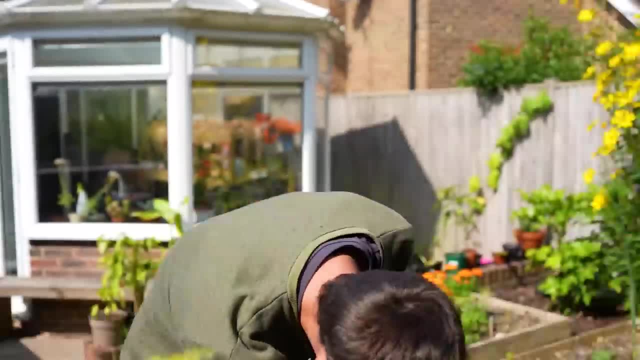 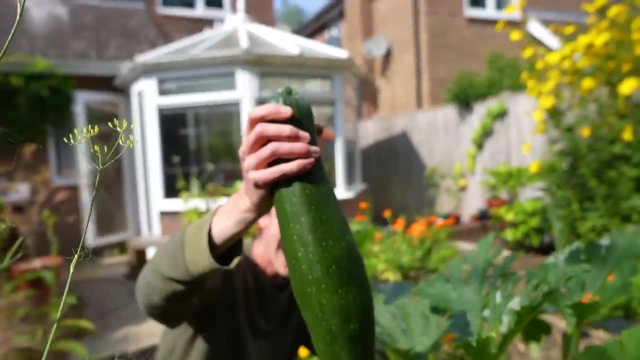 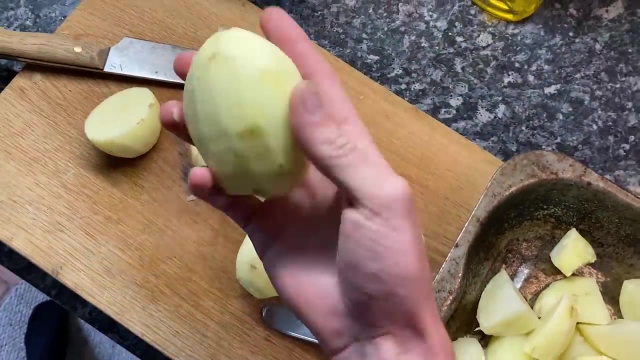 That must weigh as much as a baby. It's not even that funny. It's just Alex's laugh that made it feel. Look at it, Just been preparing some of my potatoes for roast dinner tonight. They are super fresh and they're really firm and I'm just boiling them. 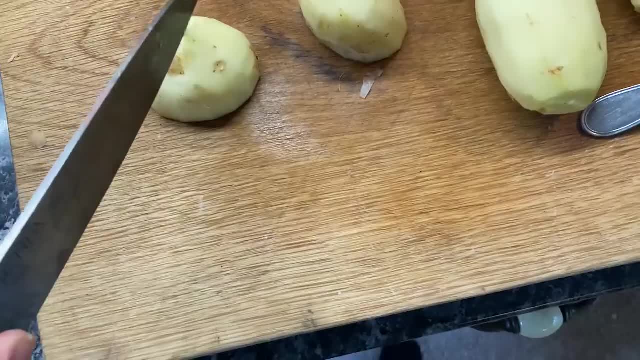 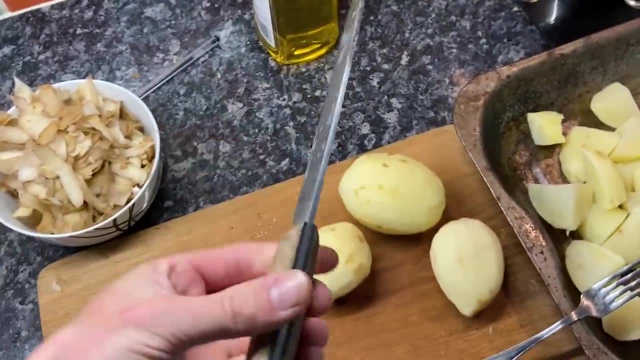 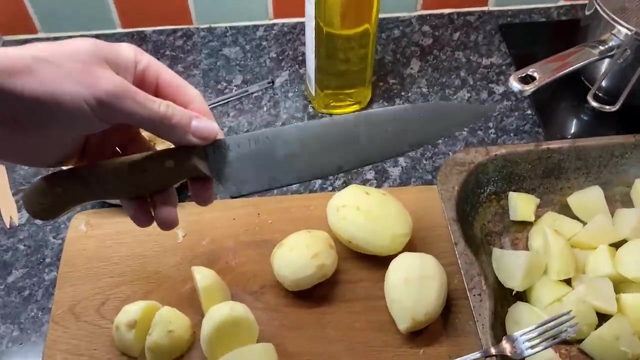 And then I'm going to roast them for dinner. Also shout-out to Mick from Brekva Knives. He made me this sweet kitchen knife, Even carved my initials into it. I've been using this for the past few months for my cooking and it's very nice. 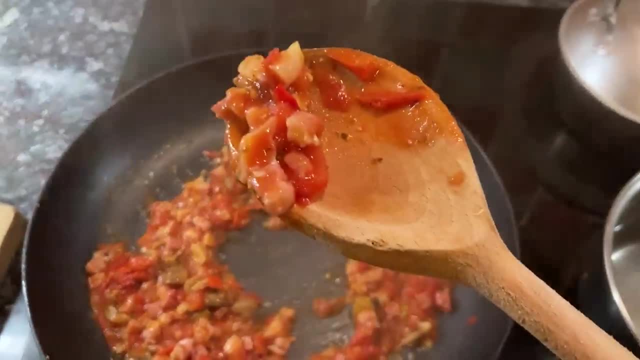 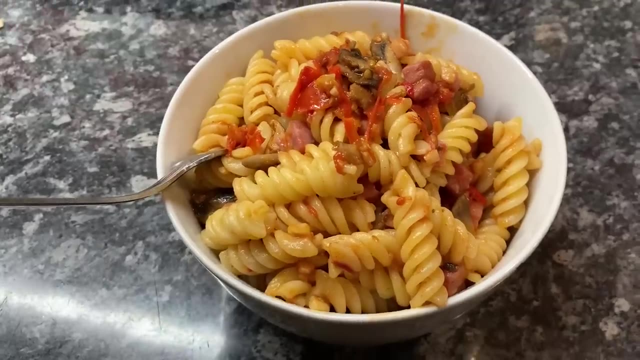 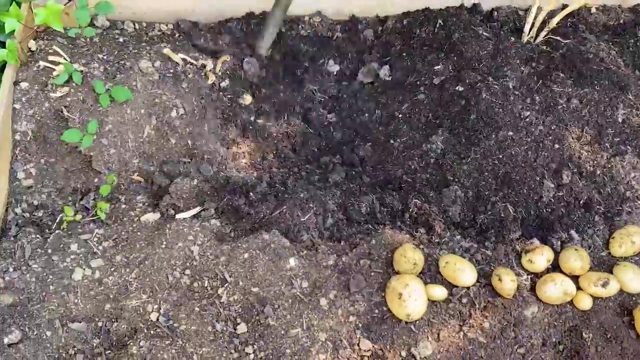 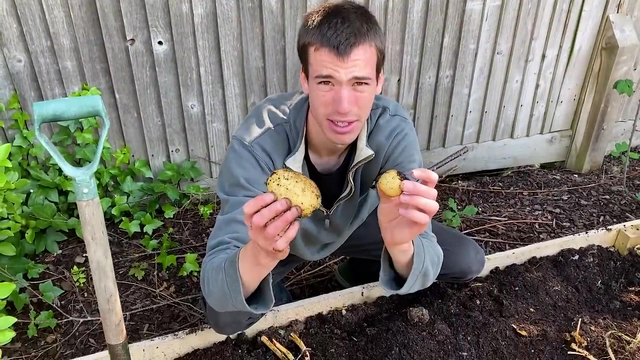 Oh, look at that, That is from my own tomatoes. Are you happy with that harvest? It's all right. yeah, I wanted them all to be this big, not that big. That was one of the last harvests of the year. 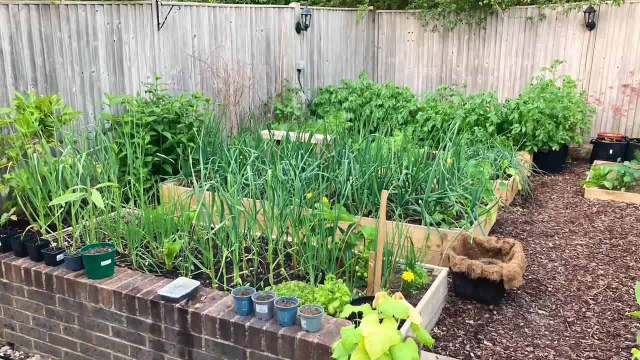 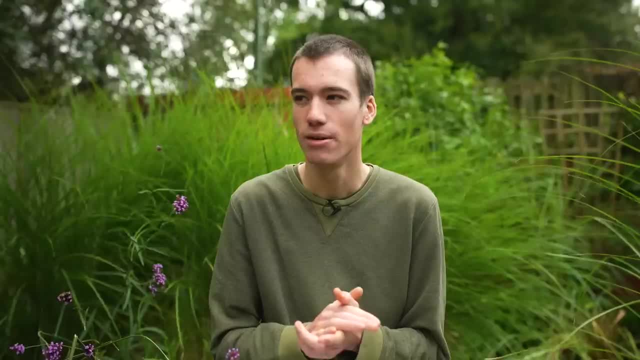 I'm quite happy with that First-year ground potatoes. So the big question is: how much food did I actually grow from my small 15-square-metre space? Bear in mind that I didn't have a clue what I was doing most of the time. 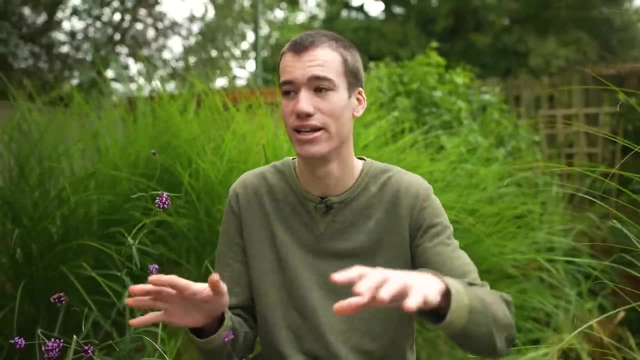 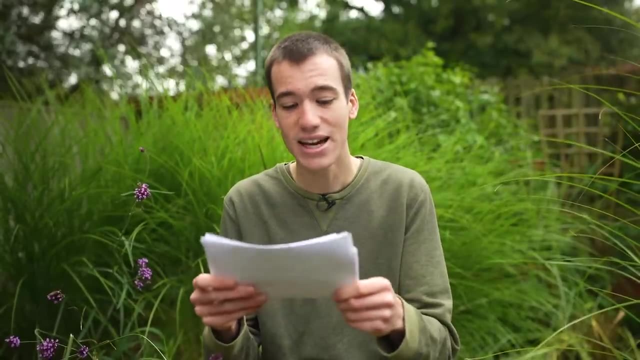 Also, was it cost-effective? Did I save money by growing food myself rather than going to the supermarket? Well, I have some statistics here, some numbers. The exact amounts of harvest are as follows: Five kilograms of cucumbers. one kilogram of spring onions. 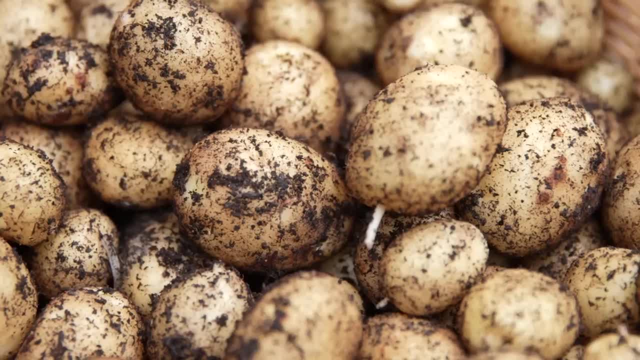 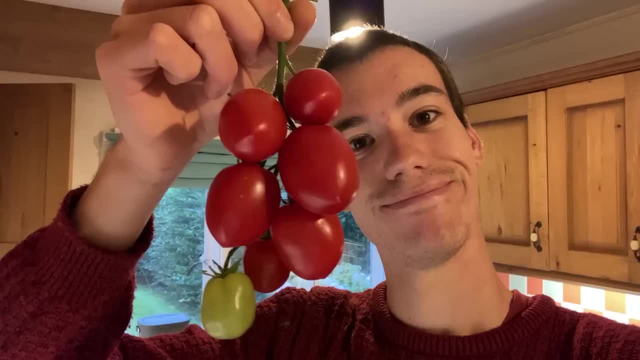 4.9 kilograms of corn, 5 kilograms of courgettes, 7.5 kilograms of potatoes, 3 kilograms of carrots- By the way, all my purple ones died- 1.1 kilograms of tomatoes. 1.1 kilograms of shallots. 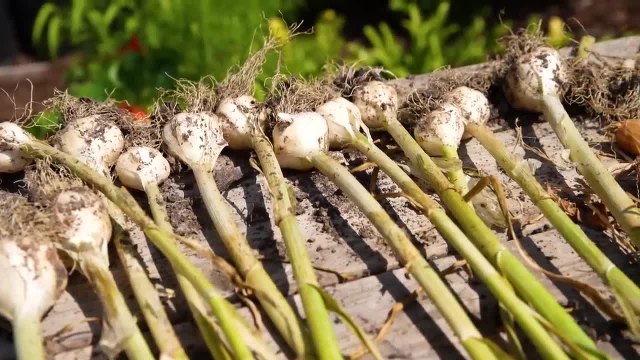 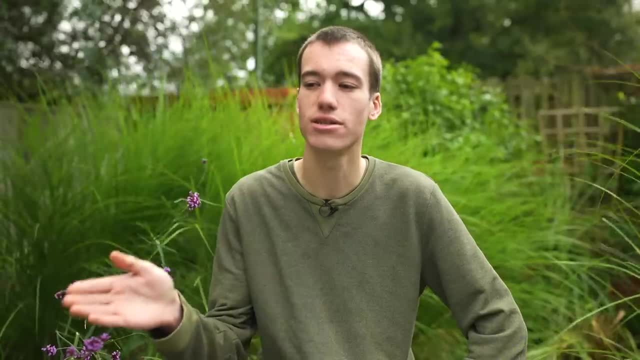 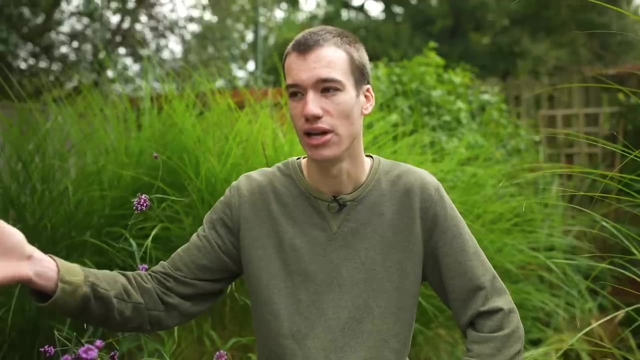 25 bulbs, 500 grams of garlic and a whopping 10 kilograms of onions, which were definitely my best crop. I looked at the prices of the local supermarkets' vegetables and compared the exact weight of what I'd grown and translated it to how much it would have actually cost me. to buy that same amount from the supermarket And I grew the equivalent of a grand total of 600.. No, I'm joking: 64 pounds of vegetables, 64 British money pounds, not weight, Seeing as I spent no less than that on the compost itself.